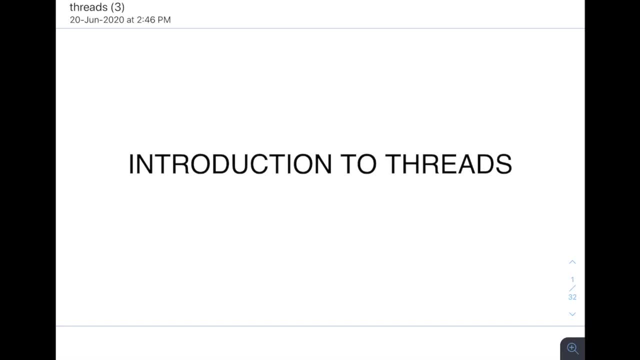 previous two sessions. I will highly recommend you to watch those Like both are of one hour each, but they cover the topic in details So you will be able to understand what is operating system, how process is managed in operating system. through my previous two sessions. 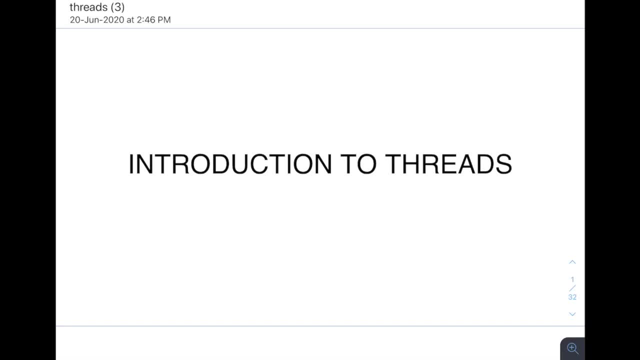 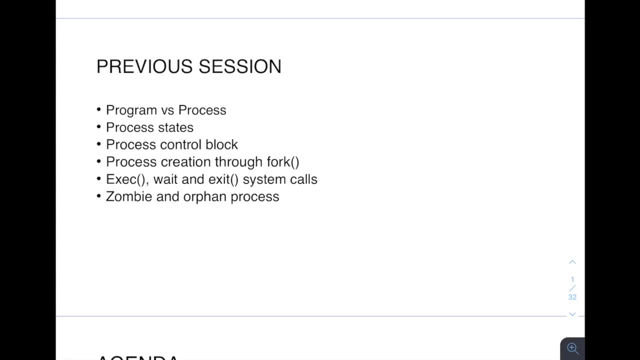 So you can find the link to those sessions in the description of this video And in this. of course, if you see a title, I will cover introduction to threads. So before I proceed, I will just request you to subscribe to my channel if you have not done so, because that 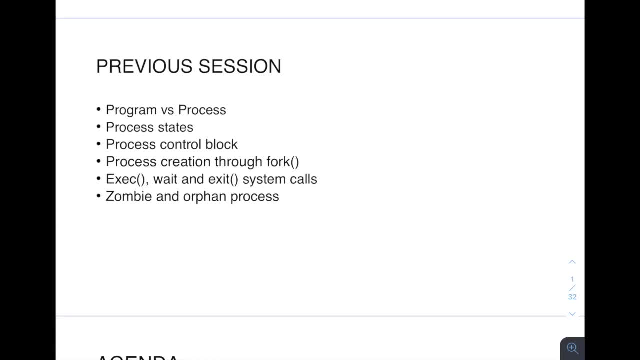 encourages me. It encourages me a lot in making more videos like this on computer science and about my work and sharing with all of you. Okay now, coming to previous session. In my previous session I covered about what is difference between program and process. So I covered about process management. In that I covered. 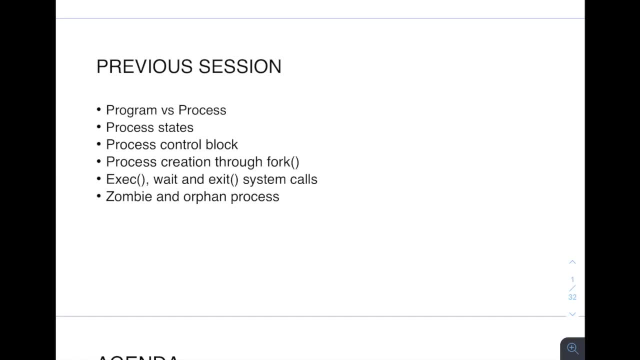 about these subtopics, like difference between program and process, what are process states, what is process control, block, process creation using through fork, like what are exec, wait, exit, system calls and, at last, zombie and orphan process. This all I covered in my last session. 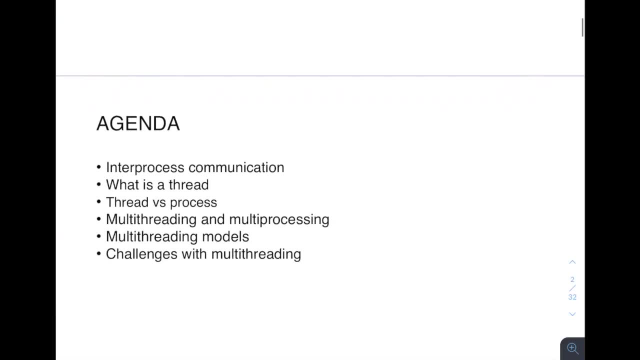 second session, And this session, like it will be like a, I will say there will be a total of 8 sessions in which I will be covering the whole operating system syllabus That can be used for your interviews, for your semester exams or for any other exams like for which you are preparing. 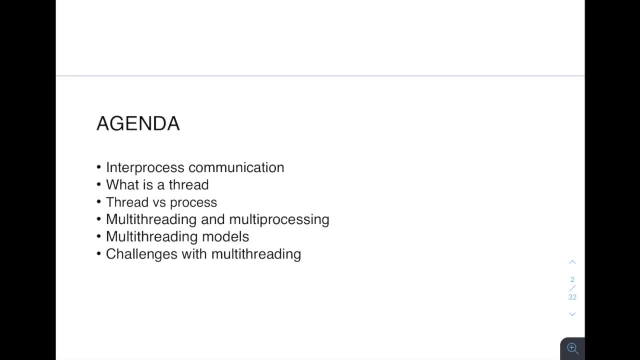 So this will cover all the basic concepts of operating system. So after you have like gone through all these sessions, you will be good with like basics of basics of opt-in system. i will not say only basics, i am also uh, teaching more than basics here, but of course you will be uh. 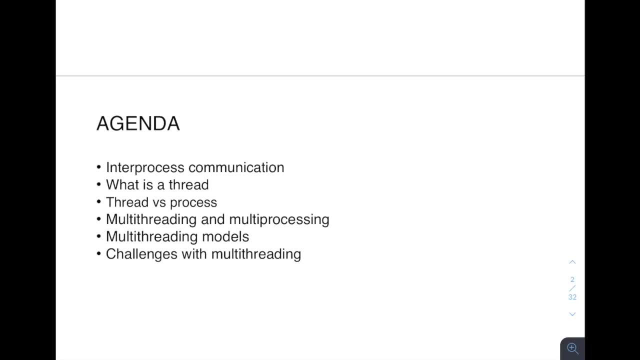 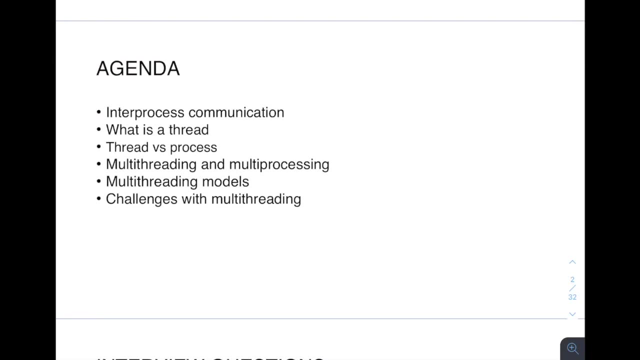 like these sessions will be enough to cover like the basic concepts. okay, the here the agenda is for this session. the agenda is like: i will start with covering the interprocess communication first, like how different process communicates with each other, then i will move to what is a thread. 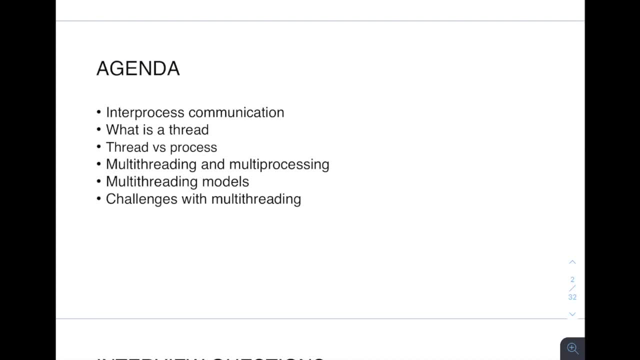 then famous interview question, that is, difference between a process and the thread, then multi-threading and multi-processing: what is the difference between this? and at last, i will cover multi-threading models and and challenges with multi-threading. what are the challenges with multi-threading? so these are all the subtopics that i will cover in this video. okay, and also. 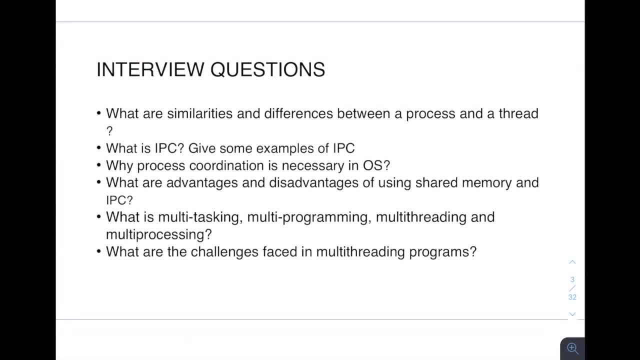 in every uh session i also cover what interview questions can be asked that are related to this topic that i am covering you in this session. so in through this session you will be able to answer these interview questions like: what are the similarities and difference between a process and the trade? what is ipc or? 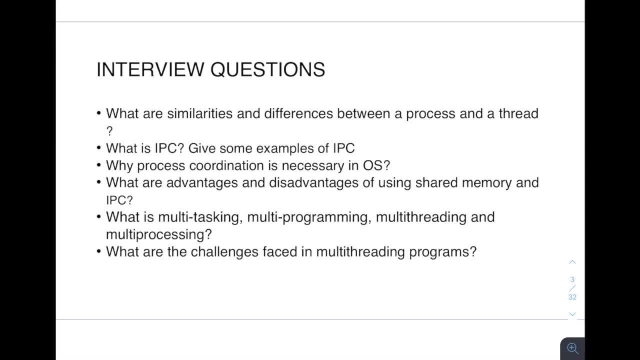 interprocess communication. give some examples of ipc. why process coordination is necessary in operating system. what are the advantages and disadvantages of using shared memory and ipc? what is multi-tasking, multi-programming, multi-threading and multi-processing? then? what are the challenges faced in multi-threading program? 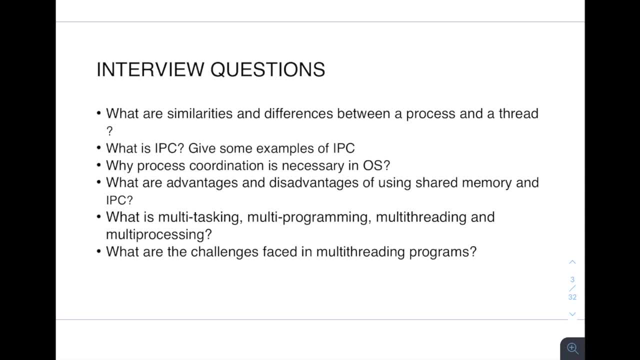 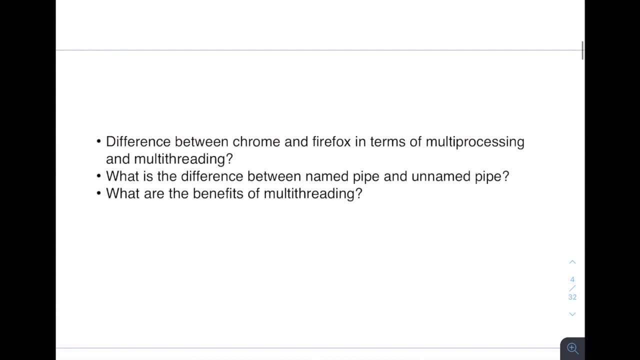 so these questions can be either interview questions or your questions in your semester exams. right, it can be anywhere. i mean, these are very basic questions for operating system. there are some more questions, like difference between chrome and firefox in terms of multi-processing and multi-threading, difference between a named pipe and a unnamed pipe, and at 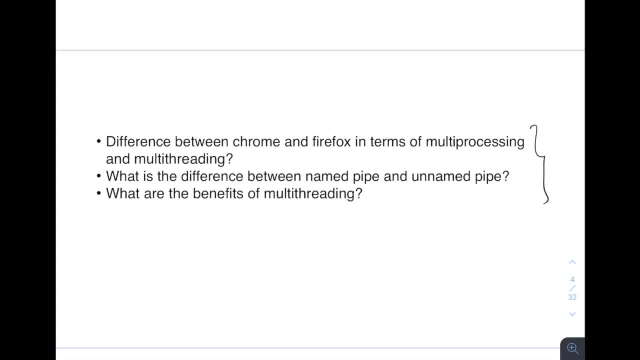 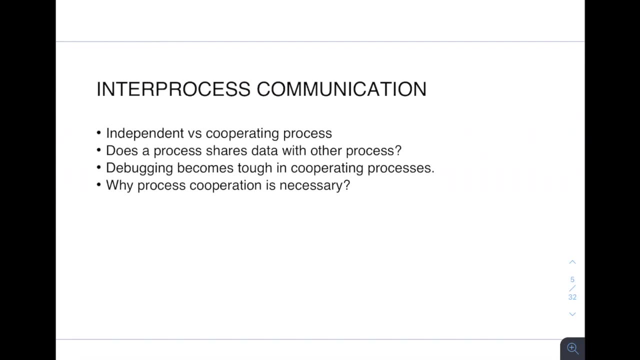 last, what are the benefits of multi-threading? these are all questions can be asked. okay, the first topic here is inter-process communication. so basically, how different process communicates with each other, multiple process, how multiple process communicates with each other. so we will look into that now. so first look at so we have two types of process. so one is 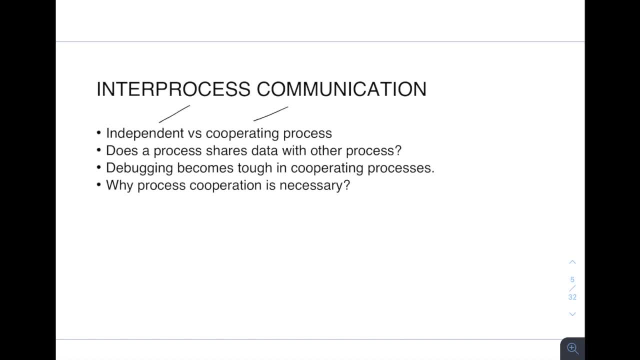 independent process and one is cooperating process. so there is difference between these two. like, independent process do not share data with other other processes, so those are independent process. they are not dependent on any other process. cooperating process are those process which are dependent on some other process because maybe they are sharing data with the other process, right? 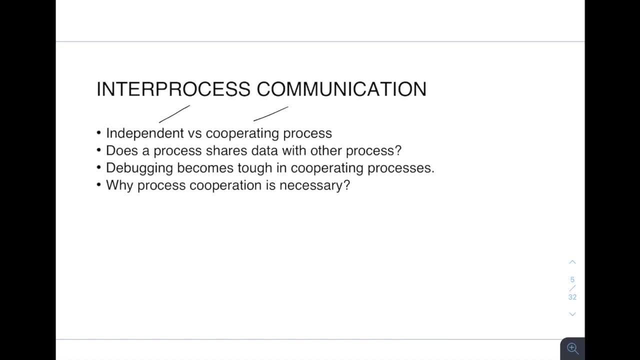 so they are dependent on on each on it for the data. so of course does a process share data with the other process. so if it shares, it is a cooperating process. if it does not, it's an independent process. also, for independent process debugging is very easier. so if you have some, 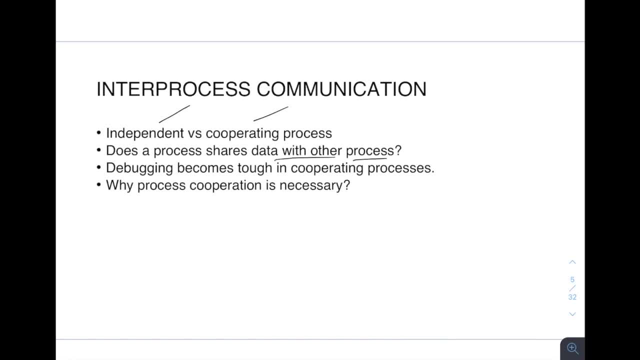 errors in the program, the debugging is very easier because that process does not depend on any other process. but when you have cooperating process, debugging may be tough because that process coordinates with other process. so you need to- i mean debugging of course can be tough- right, two processes are: 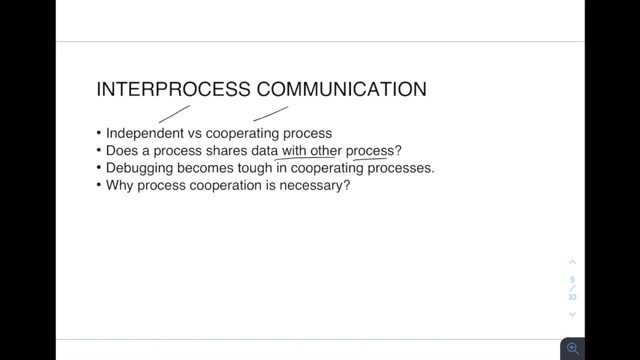 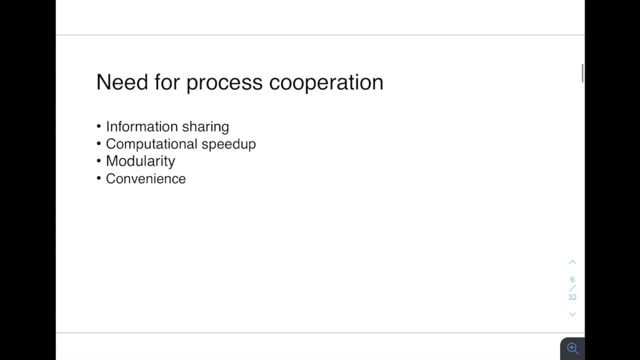 communicating here now. first, let's look at why process cooperation is necessary. so, okay, why do not we only use independent process? why to use cooperation cooperating process? right? so let's look into that. why it is necessary to use cooperating process. so there are four reasons right to use cooperative process. the first one is, of course, hash. it works and zero fuck. 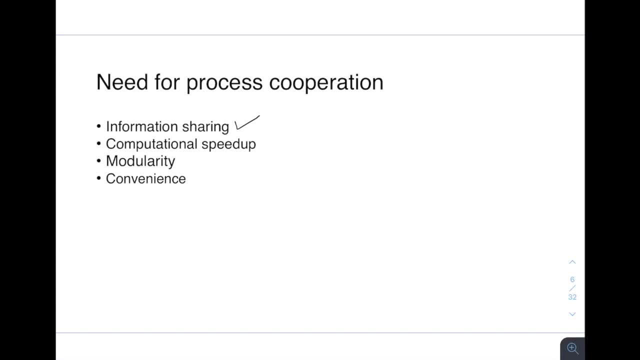 it about the operation. so first problem you have to fix is there is a there's a need for process cooperation in operating system. so the first one is, of course, information sharing. so if you have a cooperating process, they can share information with each other and that can be very useful in operating system. i will show you. i will give you some examples. 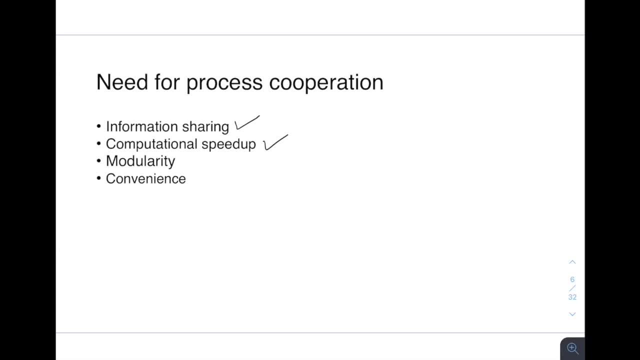 computation speedup is like if multiple process can share data. what you can do is if you're a very big program, so this is your very big program. let's say you can divide this into smaller, smaller, smaller, smaller programs, and this I mean this smaller program. let's say program 1, 2, 3. this all can share data with each. 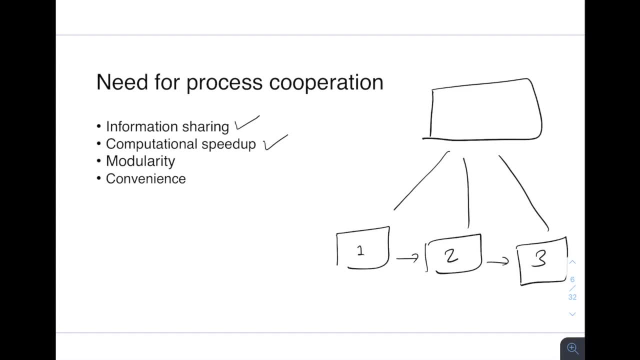 other with the help of computing process right or with the help of process communication, they can communicate with each other. now, once we have broken them into smaller chunks, now you can increase the. I mean how this? so if you, if you have run this program, single program, on the CPU, it would have taken you maybe. 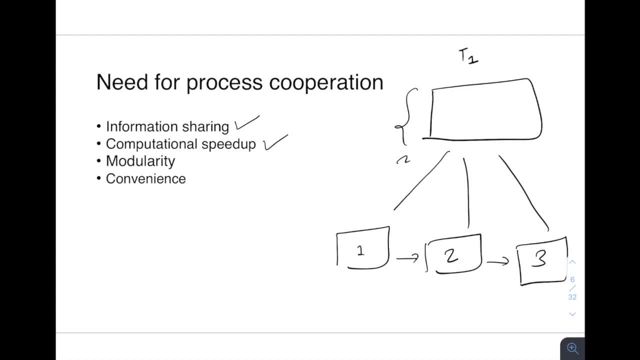 let's say t1 time. now, if you are broken down this program and you run this program on, let's say CPU 1, CPU 1, this one CPU 2 and this one CPU 3, right, then what can happen is, let's say, the time taken now for running the whole program is t2. now what? 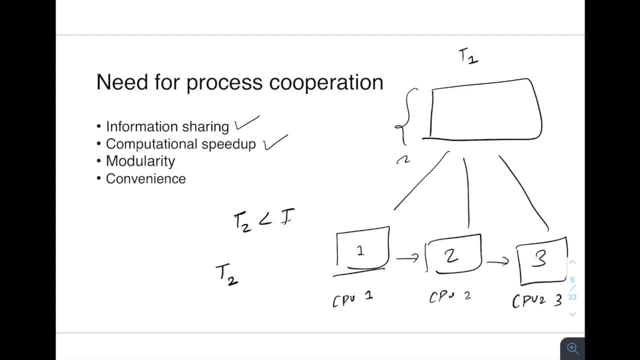 will happen. normally. your t2 will be lesser than t1 because these all are running parallelly each on the each processor now that program will finish fast because of that. that's why I'm telling: t2 will be lesser than t1 in this case and your program has basically become faster when you have broken down. 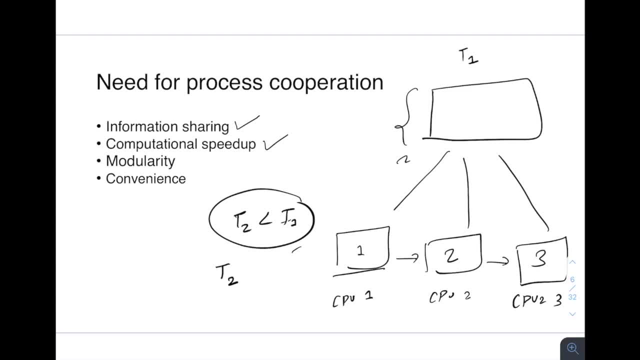 that into smaller modules, of course. the next point is modularity. so here I told you right: we have broken down the program into modules. so more modularity is of course useful for maybe computational speed up, of course. but there are other usefulness of modularity. so see if you have very 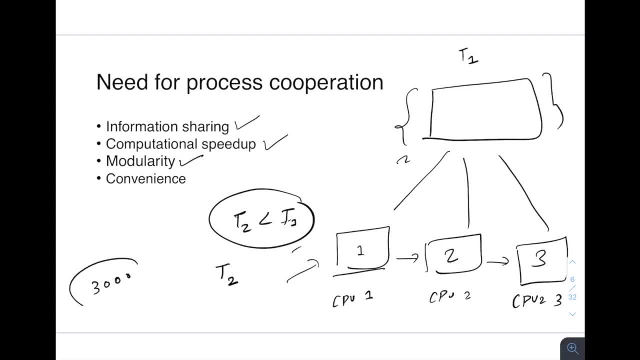 big program like containing 3,000 lines of code. now if somebody has to maybe add some new piece of code, or if if you have a new joining in your team and if you want to explain him the code, then it may become tough, because that's 3,000 lines. 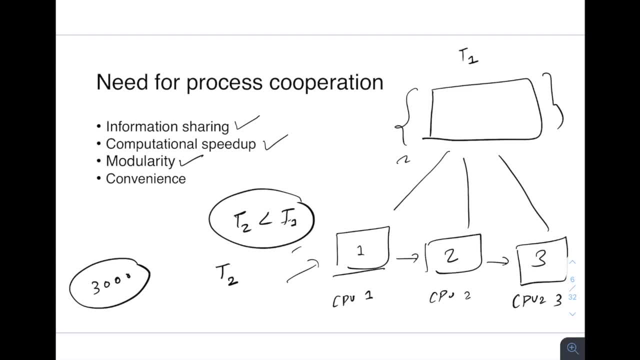 of 4,000 lines of code. but what if you have broken down into logical modules, like, let's say, the code for amazoncom? so amazoncom, of course there will be a code base for this. so what if, if you have broken down this amazoncom? 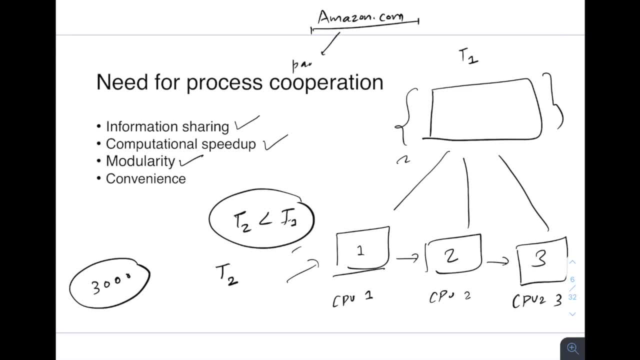 code base into logical chunks, like there is separate code for payment, there is a separate code for- maybe, let's say, checkout, separate code for listing items, separate code for showing your recommendation right. you get it like I have broken down into multiple modules and each module is very logical and 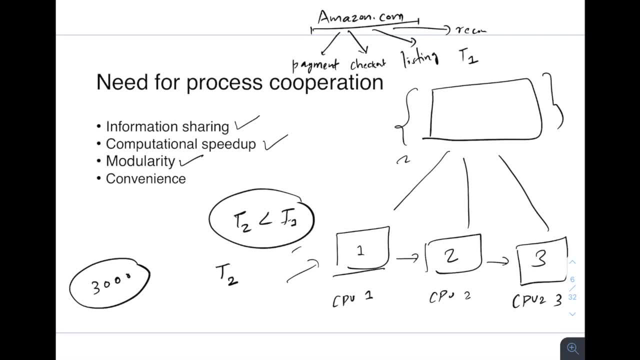 independent from other and, of course, if you want to share data among others, of course you can use- I mean, in case, let's say, they want to cooperate, of course you can use a process- I mean communication- right, of course you can use that. the last one is the convenience. so this is like: if you have process cooperation, you 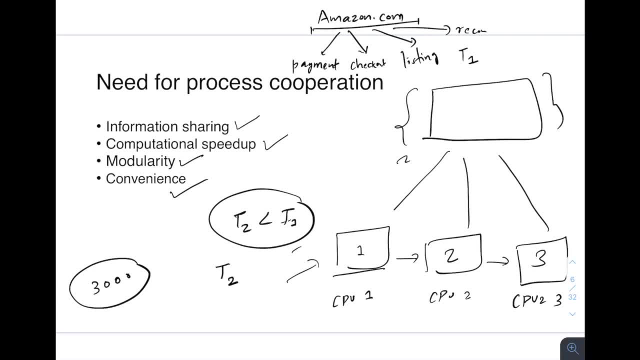 I mean, take the example of your desktop or your laptop. there you are able- because of process cooperation, you are able- to listen to your music at the same time. you are able to open a browser at the same time, you are able to do multiple things at the same time. if this process cooperation was not 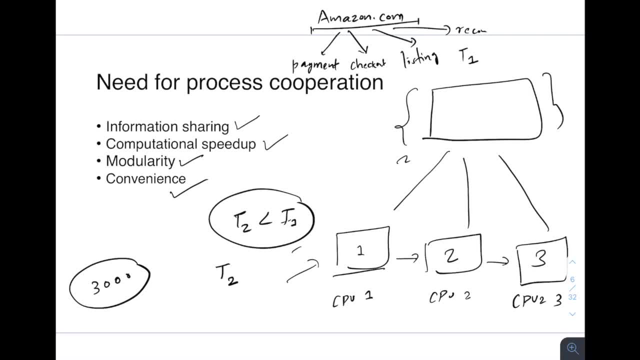 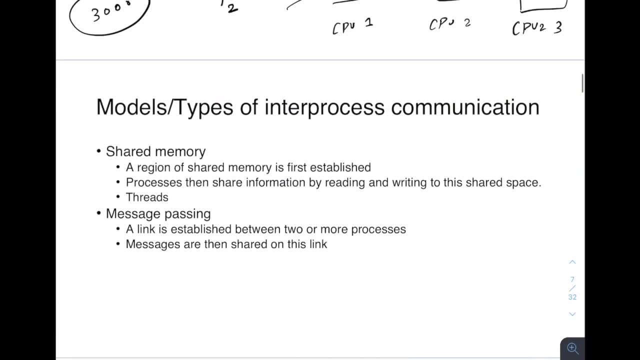 there. maybe you would not. it would not have been possible to do that, so that's why convenience is also provided when you have process cooperation. so these are the four reasons for that. so let's now look at what are the models or types of inter-process communication. this is very important. I will also give examples of 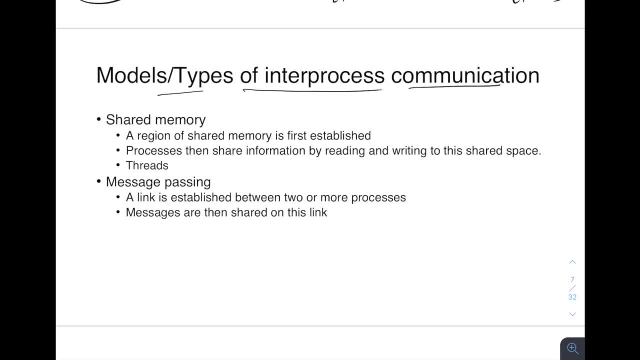 them. this is also very important. what are the types of inter-process communication? now you understood right why inter-process communication is necessary. now let's look into types of inter-process communication. first is, of course, the shared memory. so in this, what happens? a reason of shared memory is. 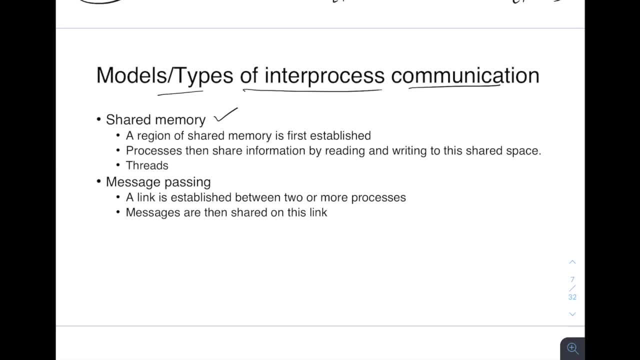 first established and once this has been established, then processes- multiple process- can share information by reading and writing to this shared space. so this happens a lot, so you will see this a lot. I mean happening a lot here, like when you use threads, right, you are actually doing the same, you are. 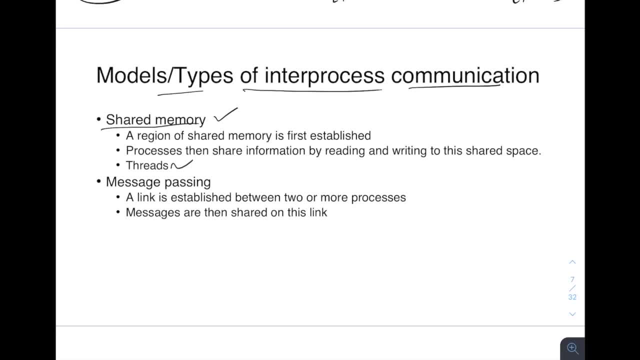 using shared memory when you are using threads. I will cover this later when I discuss about threads, but that's what you are doing. when you are using threads, you are using shared memory concept. then. the second type of inter-process communication is message passing. so in this, what happens? a link is established. 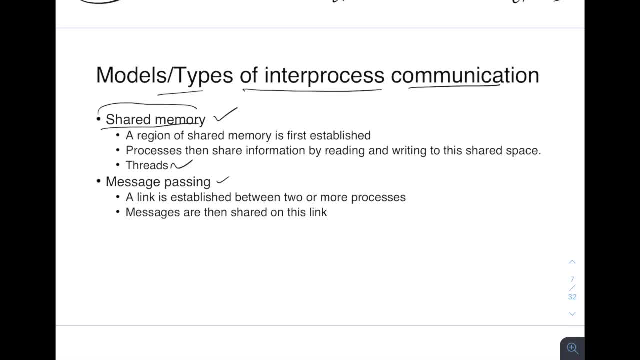 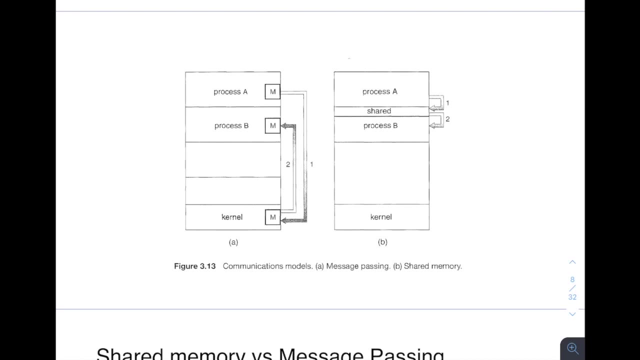 between two or more process and then, over this link, masses are shared. I will show you the examples of this, how this actually happens. you will understand clearly. here is the theory part, but I'll show you the examples also how this actually happens. okay, so okay. this is a diagram which shows actually how this 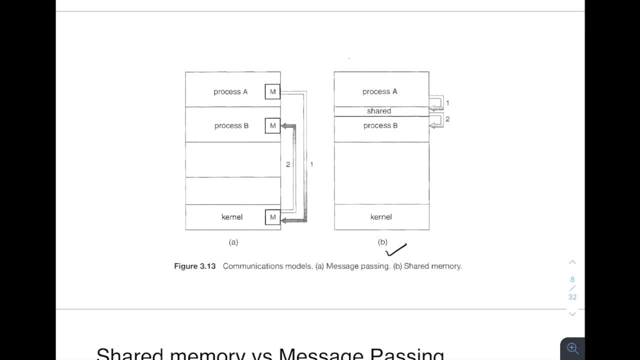 happens. so this: look at the second diagram, B diagram, which shows you the shared memory. so in said memory, if you see, this shared memory area is first established by process A and process B. after that they both can read and write to this said area. right, that's how they can communicate, like they can create a. 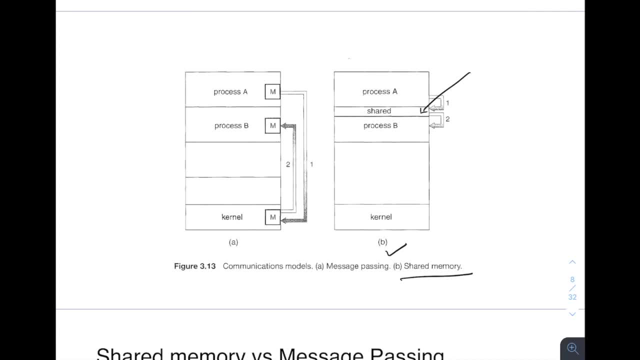 variable and they both can share the variable. they both can read to this variable and also write to this variable. similarly, both can maybe create a file and both can read from that file and write to that file. so this is this way shared memory happens. next one is message passing. in this, what happens in this case? actually, kernel is involved. 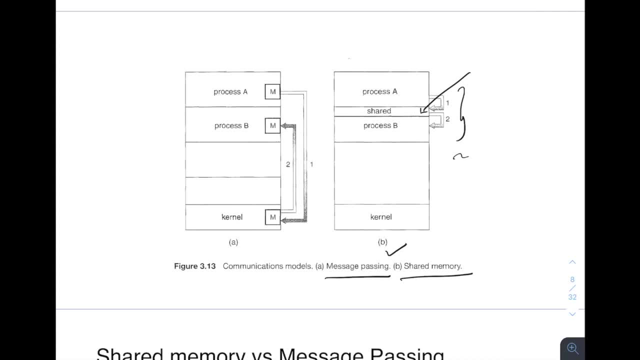 this is very important. so i am not telling that in shared memory, uh, kernel is not involved. in shared memory also, kernel is involved. so when you are creating this shared memory space, of course this is like you are creating some new memory. i mean, i mean you are asking for some memory, right, so it. 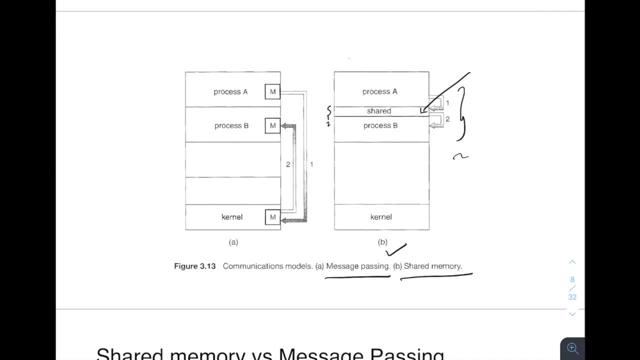 should. it is the function of kernel to do that. so of course system calls are involved. but after once you have got the memory, shared memory, then you both can write to there, both can read from there. there is no kernel involved involved there. of course, if you use mutex and other semaphore others, 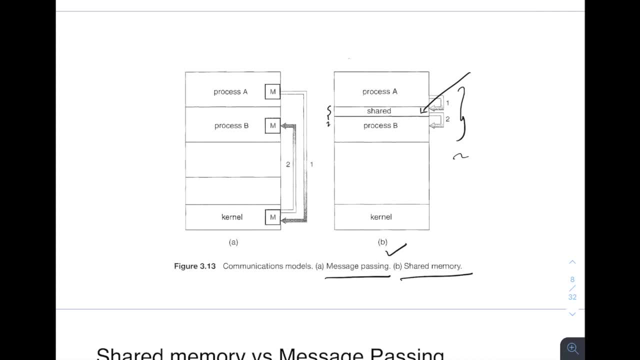 of course kernel is involved, but normally it's not involved. so when you do a thread programming, when you create the threads, okay, kernel is involved, but after you start writing and reading from some functions, their kernel is not involved. but here what happens: if you have to communicate in message passing, first the link has. 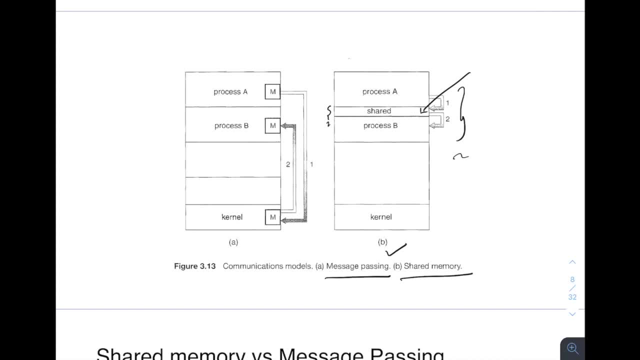 to established and then kernel will help you in, basically, communication. so take example: let's say process a wants to communicate with b so they can use some uh system calls. let's say the system calls are send and let's say receive. these are system calls that a and b can use for communicating. so what they will do is they will. 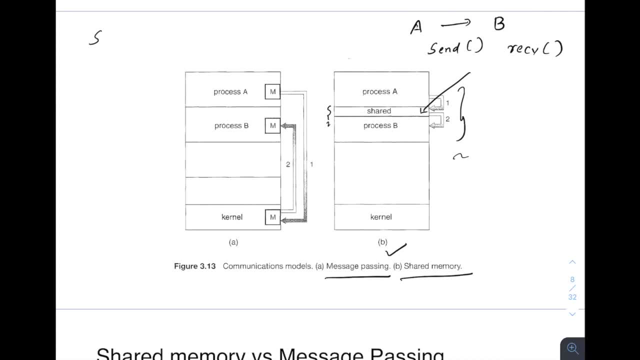 they will. so first let's say the link establishment has been done. let's say that has been done, then it will. uh, so so this is the system call that a will use. okay, sorry, not to a to b. so a will ask the kernel. okay, send this message to b, then it will go to the kernel. this system call will go to. 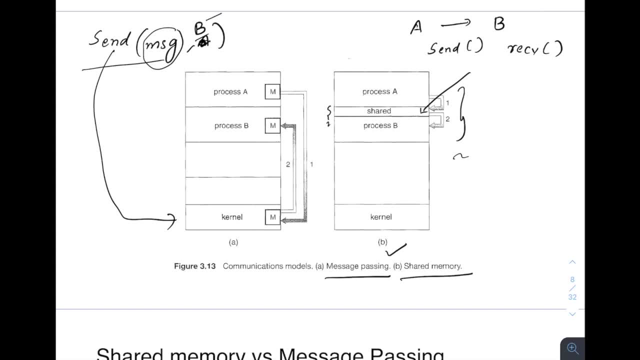 the kernel and kernel will see that this is a message and it has to be delivered to b. so what kernel will do is it will then deliver this message, uh, to basically process b and this. if you see, the communication happened right: message went from a to b. so that's how uh communication happened in. 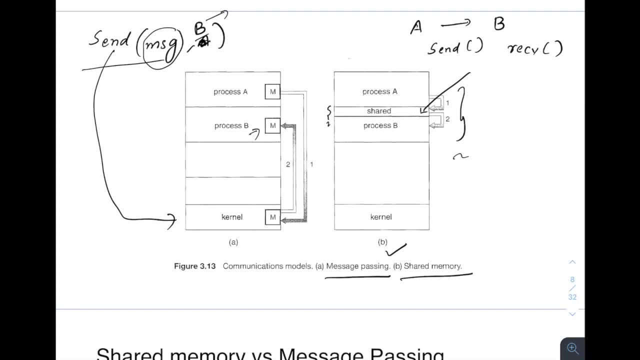 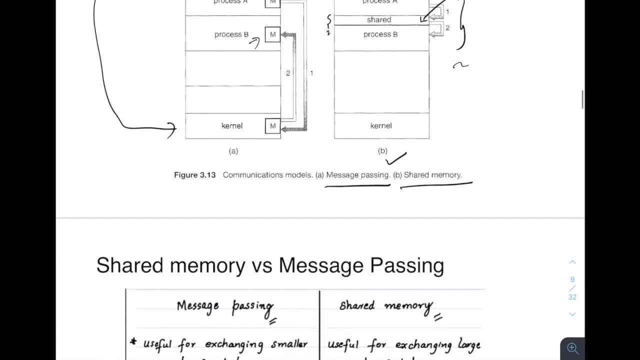 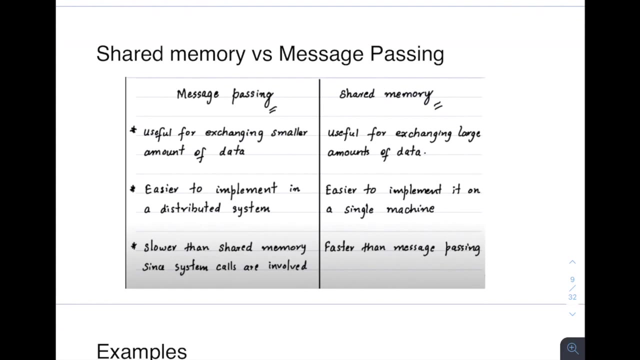 message passing and i will give you real life examples. also, because this is just a- i mean theoretical example. i will give you a real life example like how this happens. message passing happens, but before that, look into the differences between the two shared memory versus message passing. so message passing, of course, is useful for exchanging a. 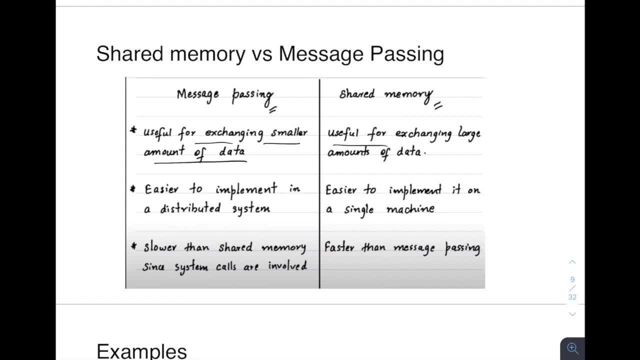 smaller amount of data. shared memory is useful for exchanging large amounts of data. this is because- see message passing- you are sending data to the kernel right and through some link and it depends on the bandwidth of that link right how much data it can handle. that's why i'm telling it's. 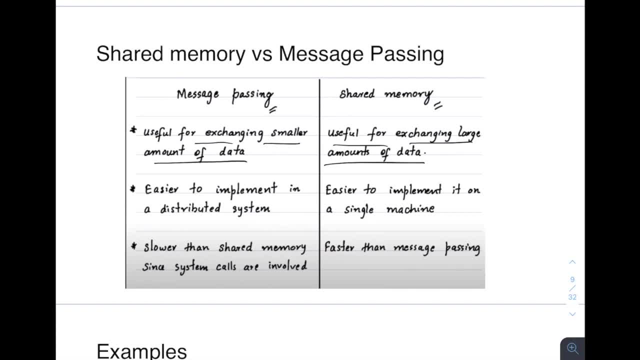 i mean, if you send a large chunk of data over that link, it may happen that the communication may become very slow. but in shared memory, what happens? you already have it, have the memory here, right? whatever data you want to fill, fill it here. if you want to like push more data, okay, ask the. 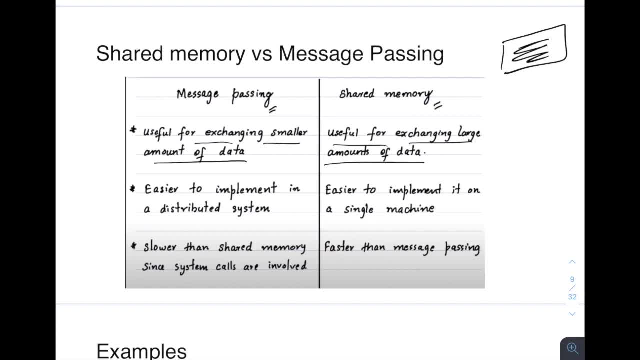 kernel to allocate more memory, right? it's very easy, right in that case, and then keep on writing and reading from this memory. that's why shared memory is useful for exchanging large amounts of data, and message passing is exchanging smaller amount of data. of course, message passing is easier to implement in distributed system. so, okay, one example of 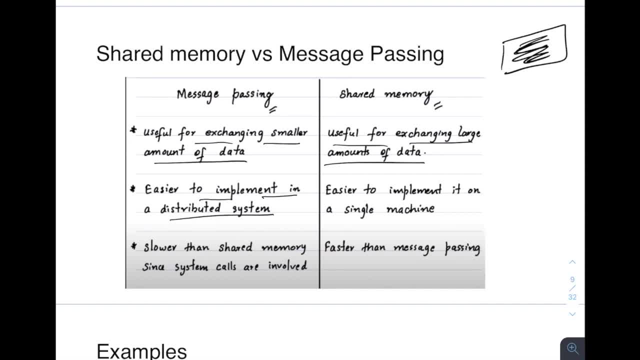 message passing is the- i mean the socket programming that happens. so how different internet devices right? they communicate with each other using socket programming like send and receive system calls. that is the example of message passing, so that normally happens on distributed system. you will have one internet device in india. other internet device can be in. 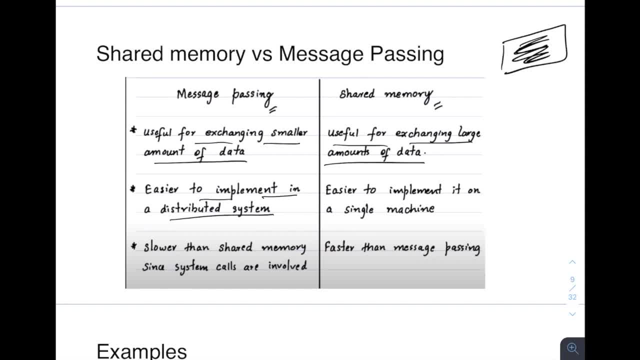 us and both are communicable and it's distributed right, distributed globally, and it's quite easy to do message passing there. but think of doing the same with the help of shared memory. right, it sounds very tough, right? how, how we can maybe i mean so you have, if you have two distributed system, one in india and one. 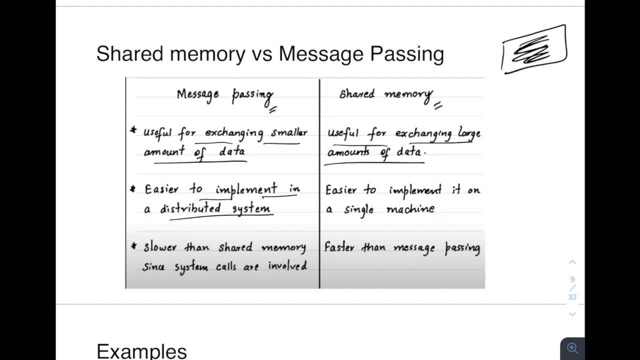 in us and you want to share data with the help of shared memory, i mean, how will you do this? i mean it's it's quite tough, right to do. i'm not telling it's impossible, of course it's possible, there are ways of doing this, but it's tough to implement. i mean this concept, so i'm not telling it's impossible. 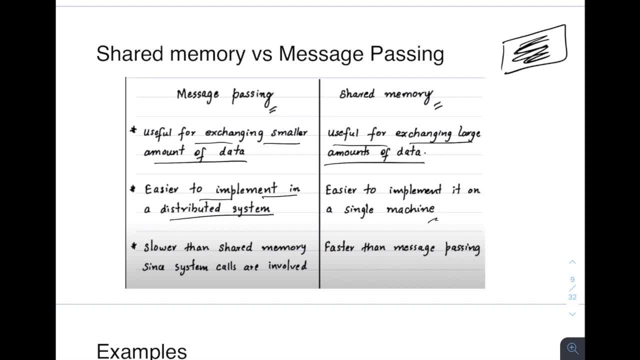 that's why i told you stuff is not easier to implement. of course, if you have single machine it's very, very easier to implement. you ask the kernel for some memory and start sharing. but how to share? i mean data on the network, right for that. message passing is uh and more easy, of course, shared. 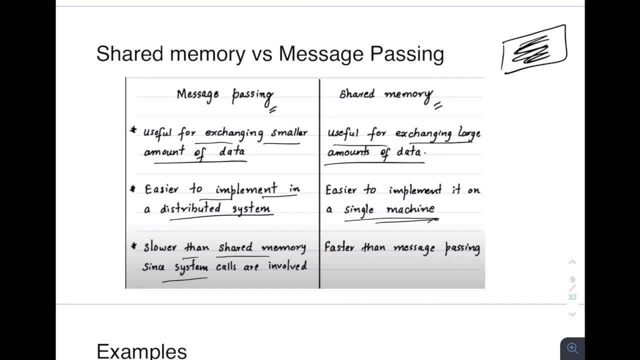 memory. sorry, message passing is slower than shared memory because i told you, system calls are involved in message passing. every call has to go to system call, then system call will, and that's kernel will then deliver the message to the other process. that's why this is quite slow, because 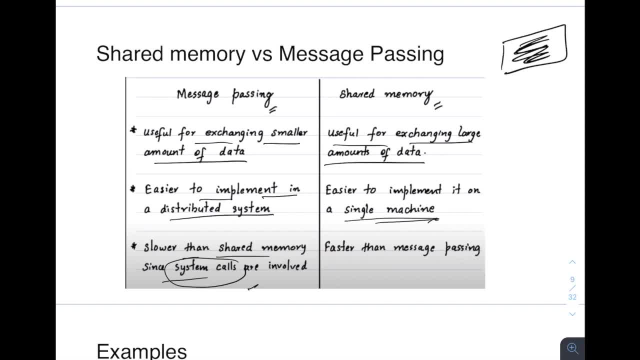 you are involving kernel here and kernel will take some time. of course, this is faster than message passing, because when you are reading and writing to the shared space, mostly the kernel is not involved in that case. now let's understand more this with real life examples. so, of course, 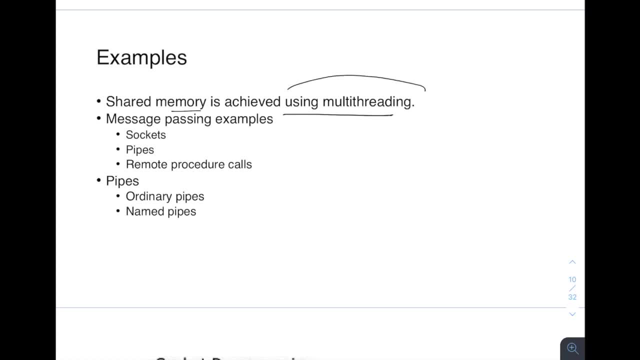 shared memory is achieved using multi-threading. this is one of the way of using what i mean achieving shared memory. that is, multi-threading programming. in multi-threading, when you have multiple threads, all the threads will share a common piece of memory and they both- all the threads- can read and write to this memory. so that's shared memory. very simple example of 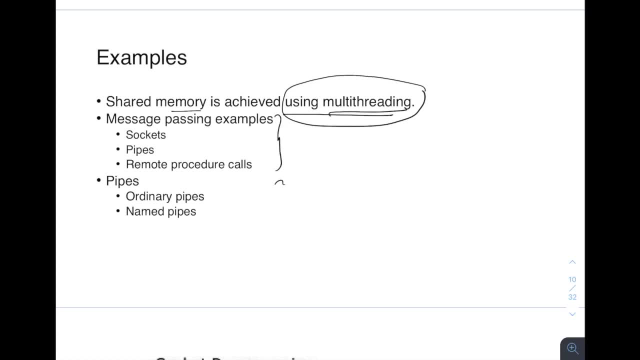 shared memory for message passing. you have some examples like sockets. i told you about sockets. right socket is a famous example of message passing- socket programming that you do. pipes is there. i will tell you more about pipes in the rails after some time. and also you have remade remote procedure call. i will not discuss much about remote procedure call. 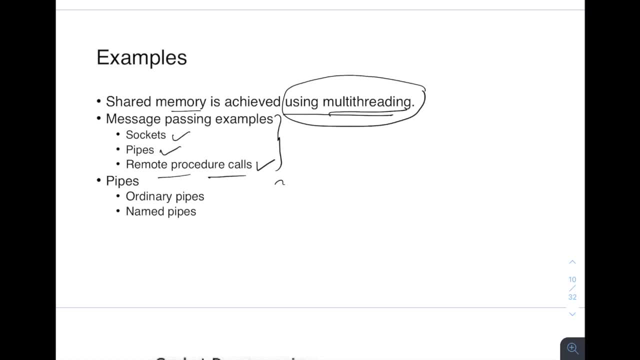 here, but they are similar to socket programming. i mean you are communicating with some other devices, mostly in rpc also. then you have pipes pipes. there are two types of pipes, actually: ordinary pipes and named pipes, or this: ordinary pipes can also be called as unnamed pipes. so basically you have two types of pipes: unnamed pipes and named pipes. okay, let me uh dive into. 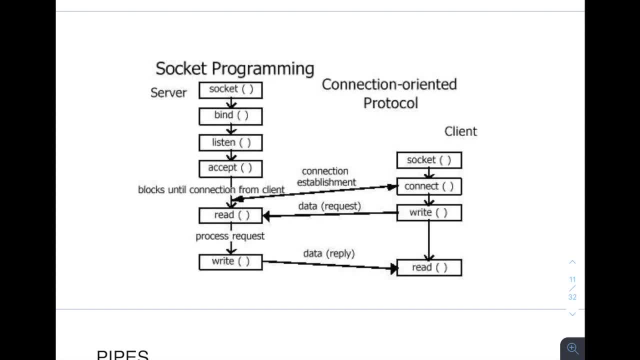 this in details so you understand these real life examples better. so socket programming: if you have not done socket programming, maybe if you are in third semester, fourth semester, right, maybe you have not taken a network networking course. okay, you will not be aware of socket programming. but this socket programming actually helps in, like whatever the communication is happening on the 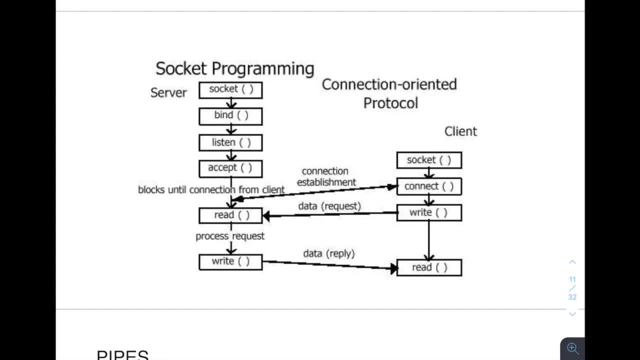 network or the internet. that is done by the help of socket programming, where you bind a socket- sorry, you create a socket first, then you bind the socket, then the server listens on the socket, then the server accepts a connection from the client. so you have client and server model. so client is basically you and the server is like google server. 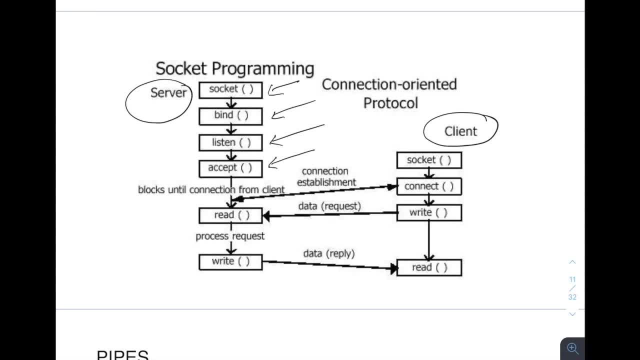 or linkedin server which is basically, uh, somewhere in us or some other countries. let's say, then, now you will. basically you are, you will. i told you first the first thing is to establish a connection. so you will first establish a connection with the server. so once this is done, you will send a data. 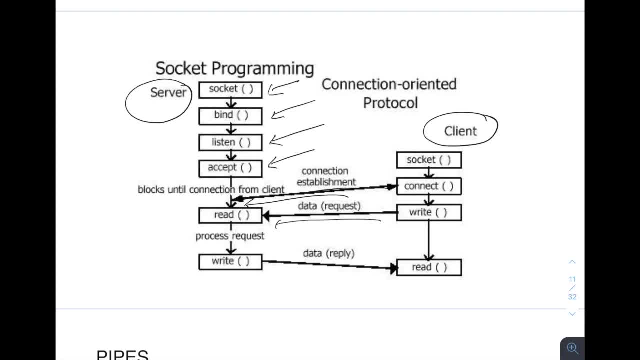 request, like you will say that, okay, your browser will basically send the request, so your browser is not gonna contact us. send me the google page. send me the page for home page for googlecom. this is the request and this will be normally done with the help of, i will say, a read system. call right. 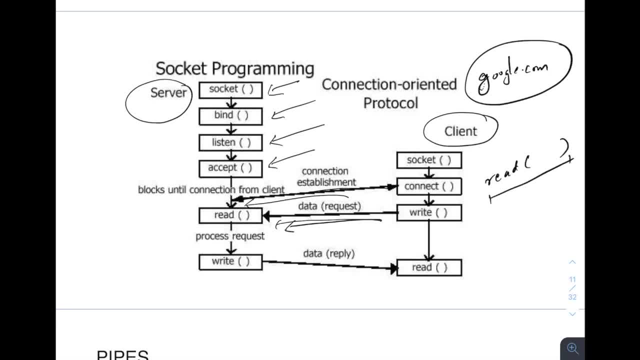 read system call, it will be: uh, you will be used. and then what will happen once the request will reach the server? it will process this request and it will use the right system call and it will reply with this, with the right system call, and it will basically travel over the network and reach. 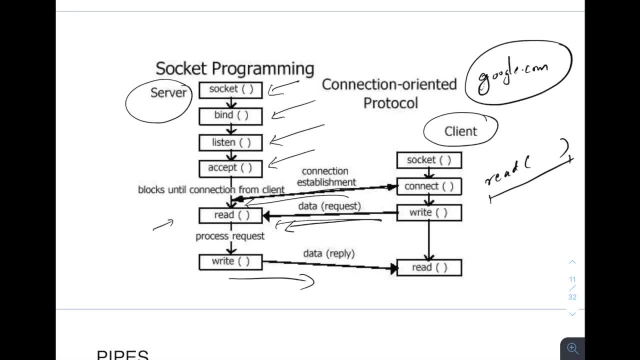 your browser basically rendered that home page on your browser. that's what happens. this is a famous example of message passing. so if you see, message message was extend, right, so what is the message here? so the message here is the googlecom uh html page that was transferred, transferred from here to here. 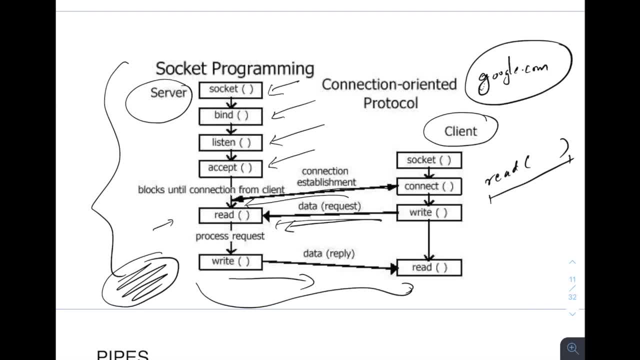 from server to client and also one message also: this data request also got transferred from client to server also. that is also a message. so this is like okay and okay. you will think how i am telling. this is process communication, interface communication, because this client is actually running some process. the browser is still a process itself. right, the your browser. it is. 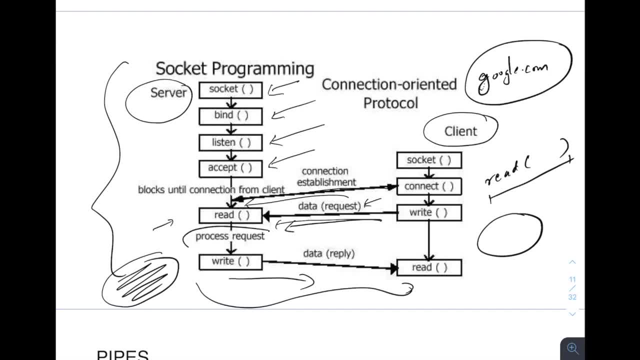 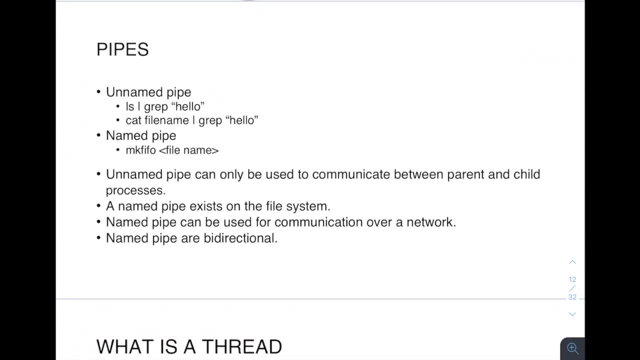 it's still a process. here also somebody is processing your request. that is also a process. so that's why i am telling process communication took place here, or interface communication. another famous example is pipes. so if you are using terminal a lot, you, you, you would have used uh, pipes, unnamed pipes, a lot like this command ls. 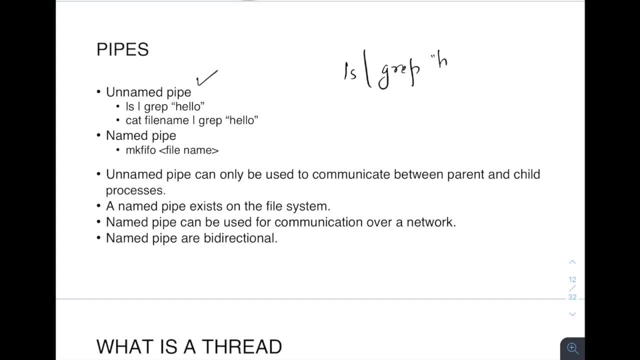 then grape hello. let's say this is. i'm giving you some simple example. so this will basically search your all the files in the current directory directory and uh, give the output the files that have hello in that file name. that is hello. other can be like cat file name. uh, grape hello. so this: 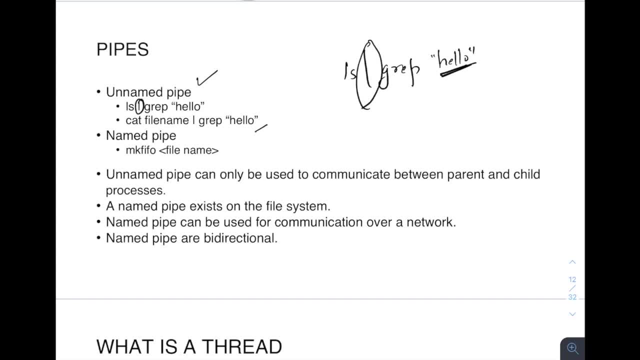 is: this is actually the pipe operator, this one pipe operator. this is the pipe operator actually. and what is pipe pop? okay, you will think how enterprise communication is happening here. see, this is happening. something like this: ls is a command which you are running now. it will, uh, basically. 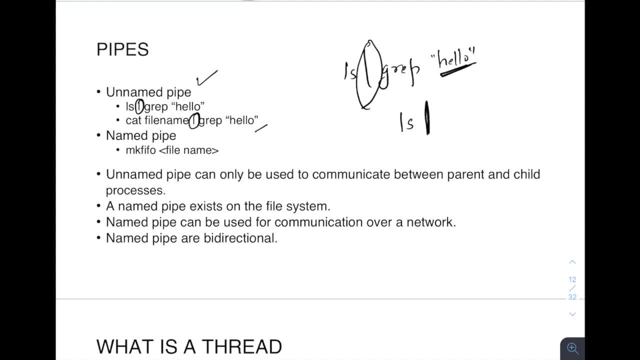 output something right now. if you use the pipe operator here, the output will be passed to the next command that you are writing here, that is grape hello. so basically what happens, ls is also a process or a command, so this is actually process itself. grip is also a process. now you want to pass. 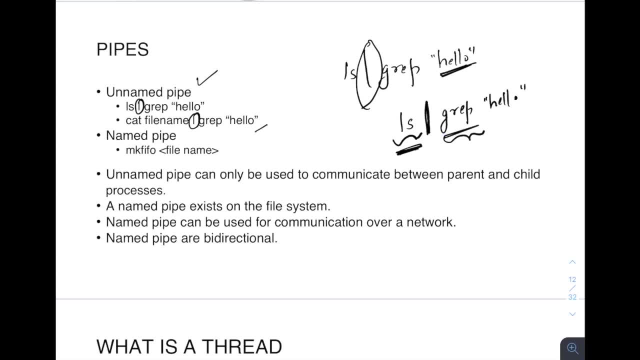 ls command to grape command, right. so output of ls command should be an input to grape command. now, if you use the pipe operator, this will help in passing that. so that's how. that's why i'm telling here again. internal communication took place. the output of this uh was transferred to. 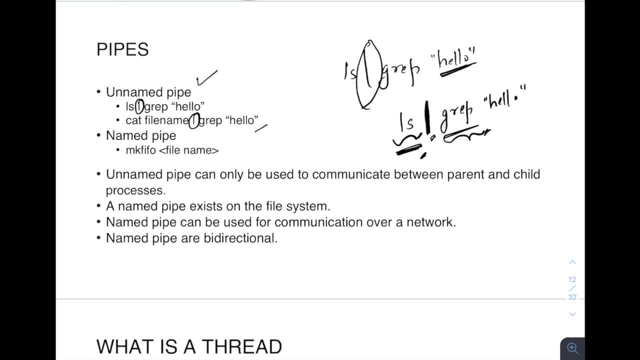 input of grip command, of course, other than you have. so this is uh, unnamed pipe. then you have named pipe also. so the issue is okay, i will discuss that. so in named pipe, what you can do in linux, you can use make fifo command, mkfi, fifo and file name and it will create a name pipe and i will discuss. 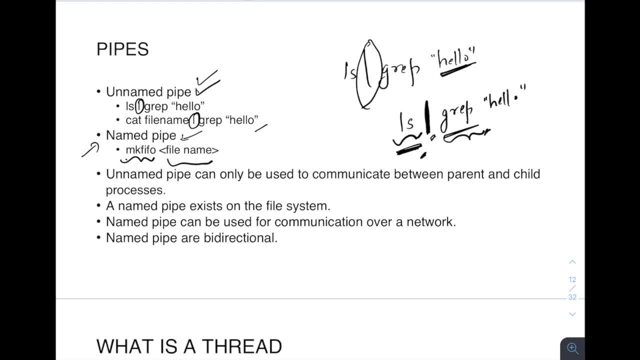 the difference between name pi by unnamed pipe. so unnamed pipe can only be used to communicate between parent and child process. so ls is the parent process here. right, you are passing the output of parent process to the child process. that is great process, but it is not with name. 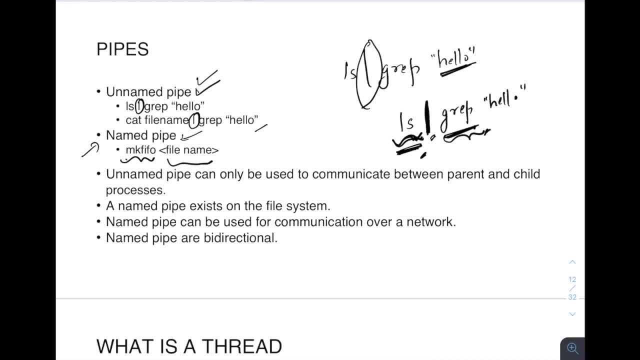 unnamed pipes in name pipes. so let's say you have created a named pipe. let's say, and the name is named pipe, so this is basically a file that is there on your disk. this is the pipe file that is there on the disk. now any process. so this is basically like a fifo queue. so you 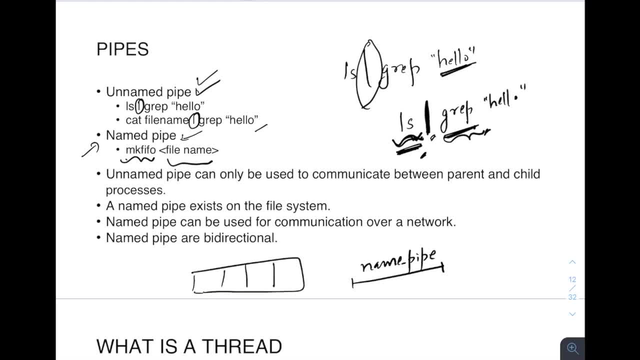 have basically a fifo queue kind of thing, and now any process can read to this or and any process can write to this. there is no, i mean limit on this, like, okay, only parent can pass the output of child or something. any process can read right to here and any process can read from here, so that 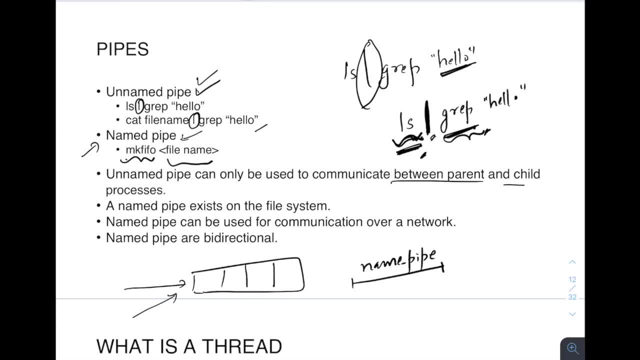 difference is not there? this difference here. also, a name pi exists on the file system or it's permanent on the disk, on your disk. this is not with the, this unnamed pipe. once you have run this command, the pipe disappears. right, it is not permanent, but these name pipes are permanent. 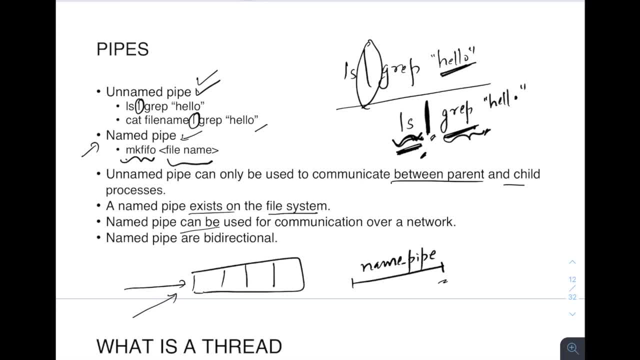 on your disk. also, name pipe can be used for communication over a network. so if you host this name pi file on your network, then of course you can communicate it on the network also. right again, name pipe is bi-directional. if you see, this is unidirectional, right? you can only pass the ls. 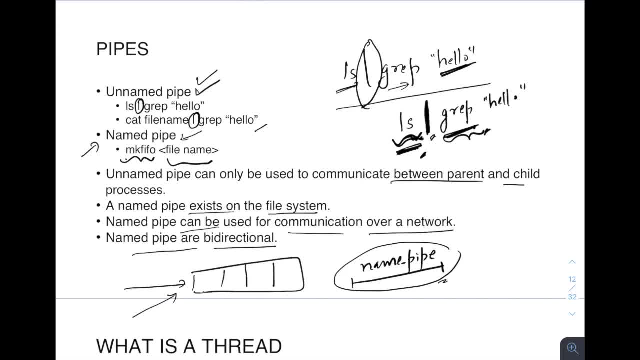 command output to grape the reverse. you cannot do here right. but in this case named pipe is bi-directional. i mean you can also read and write from this. both you can do in named pipe. you cannot do the same in unnamed pipe. so this is all about interposed communication and i have given you the 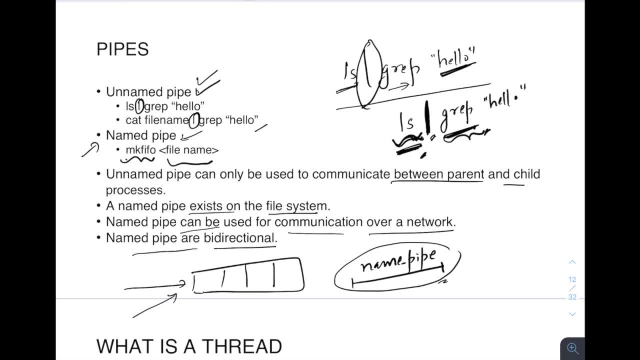 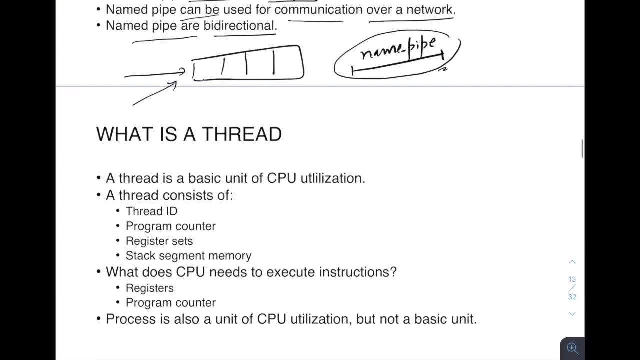 theory of like. what is difference between? i mean, what is interposed communication? what, what is the types of interposed communication? and i have given you a lot of examples here to show you, like, how interposed communication work. now you should be clear with these concepts. now let's move to the second part, that is, what is a thread? we will discuss about multi-threading. 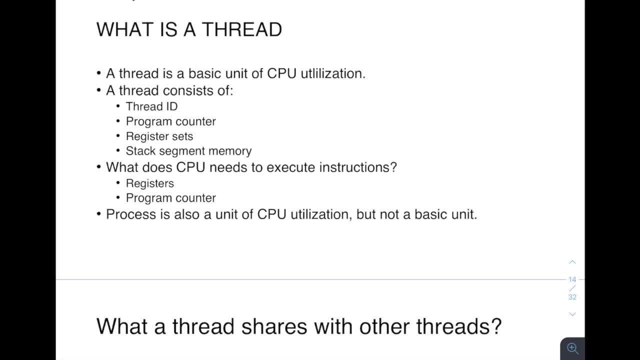 multi-processing here in details. so a thread is a basic unit of cpu utilization. this definition is very important and this makes sense a lot. let me explain you how this definition works. so let's go to the first part. so let's see what does the thread thread consist of? a thread consists of thread id, program counter. 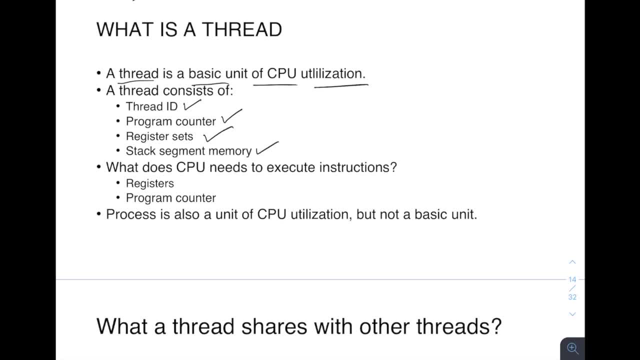 register sets and stack segment memory. normally these four are the uh important parts of a thread. now think about this: what does cpu need to execute instructions? so cpu needs actually registers and program counter. and this program counter is also shooting some registers. so normally the cpu needs like registers to uh. 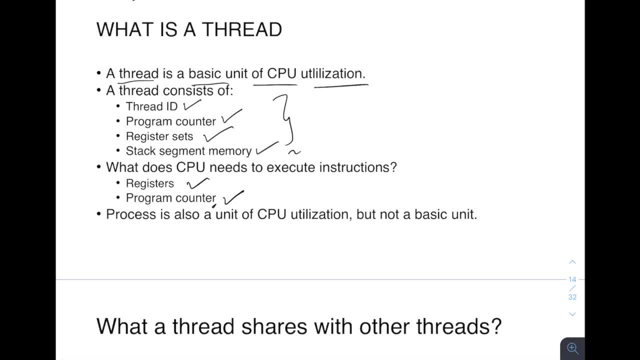 execute instructions- right. but think about a thread and, uh, cpu, right. so thread also has all of this, uh, all of the data that is actually used for i mean executing instruction on the cpu, this, it does not contain other information. it only contains the information that is needed to run the program. 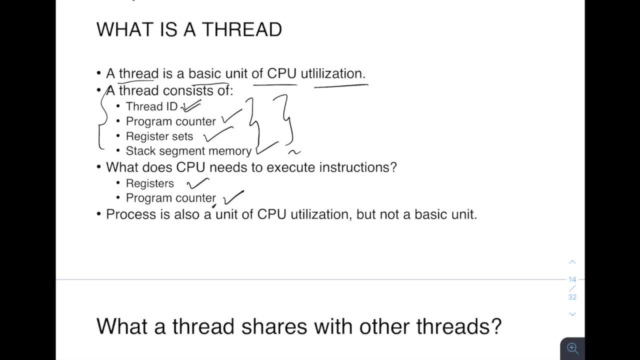 or instruction on the cpu. so of course leave thread id. but this program counter register sets and stack 7 memory. these are very useful for running an instruction, so that's, that's why it's a basic unit of civilization. so this process, process is also a unit of civilization, but not a basic unit, because the process contains a lot of other. 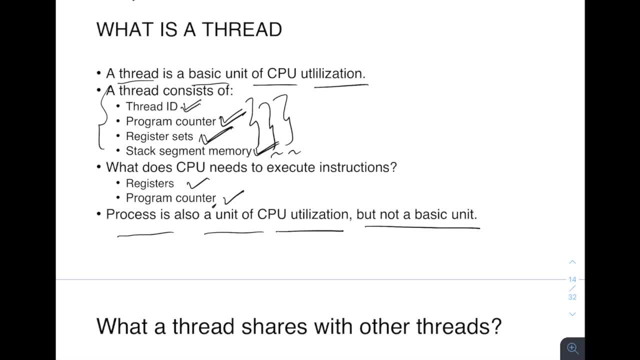 information also, like: what are the list of open files? uh, what i mean. also memory, uh, information about uh like heap memory, data memory and and all this memory right. so process contains a lot of other information also, but thread only deals with these four: information mostly, and cpu also. 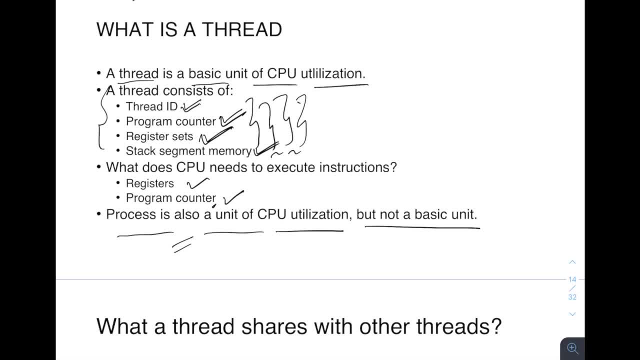 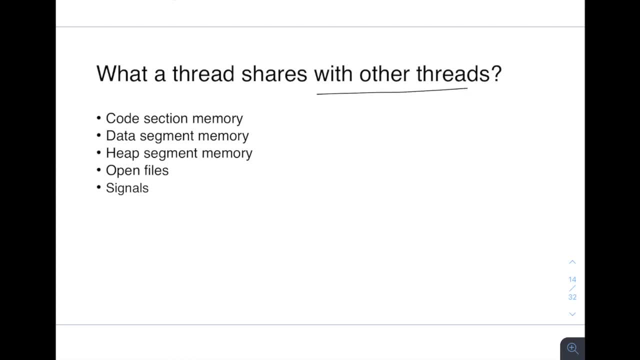 and it begins on week three. second, are mainly related to your cpu module right. extraordinally, however, when you run it, fruit object itippu- behold is a basic unit of speedYes, itettleilization. now let us understand what a thread shares with other threads so different. we process 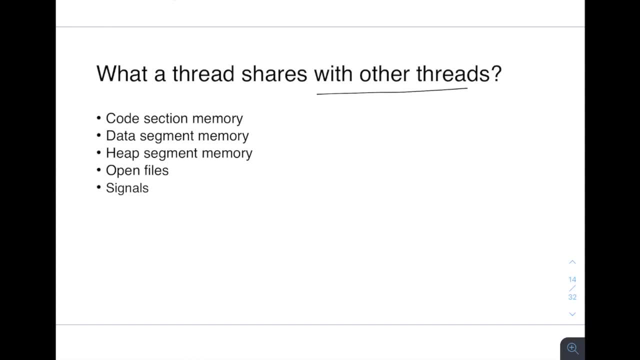 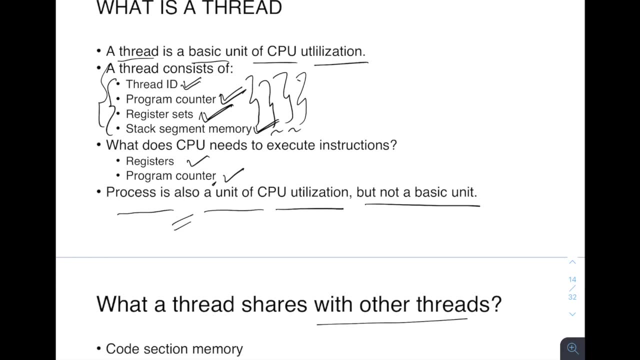 and thread, in the sense that a thread shares some data with other threads. so, of coursethis four are unique for threads, butthey also share something, so that this four will be unique for each thread. the fourth thing, butthere are other things that they will share, like code. 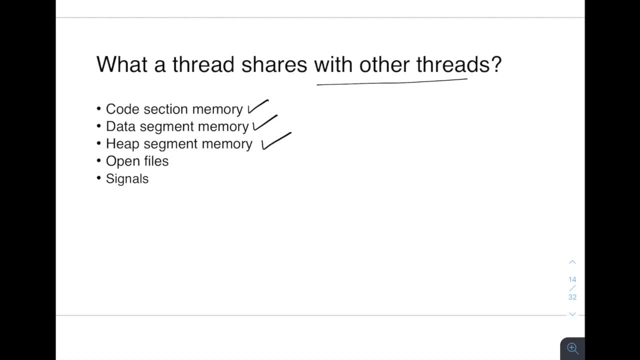 section of memory data, segment of memory heap, section of memory, open files, signals. so this all they will share with other threads. so this is very important to understand. so that's how they differentiate between threads and the process. a process does not share all of this with other. 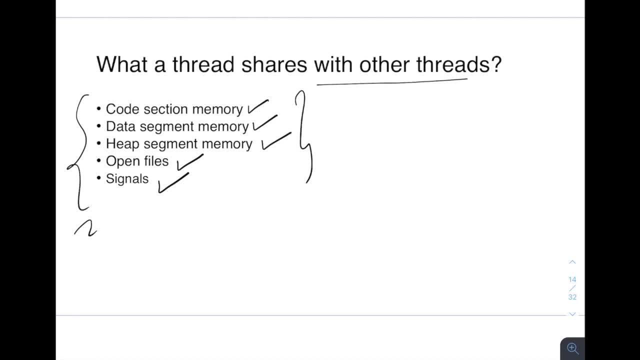 process but a thread does, so that's a very that makes a huge difference actually. so, basically, if you see, the difference is that threads share a lot of resources with other threads but process they do not share resources with other process. so, within process, if you have two, process both. 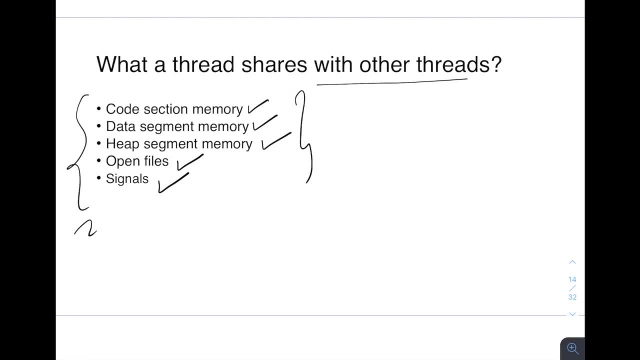 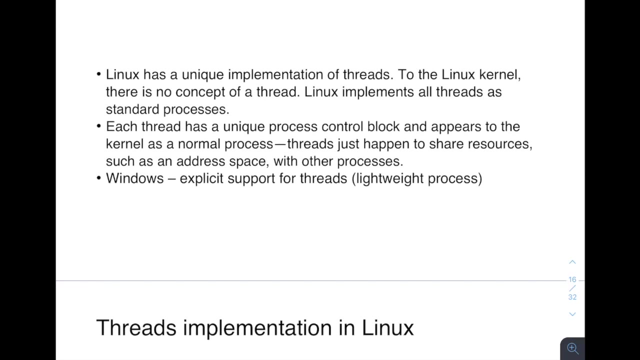 the process will contain like separate code section of memory, separate data segment of memory, separate heap section of memory, separate open files, separate signals. but if you have two threads within a process, both will share this file and also. uh, okay, this is just some i will say extra. 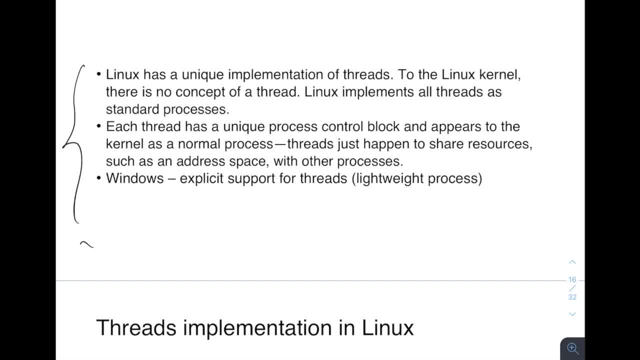 knowledge. uh, it's okay- good to know about this- how linux actually implements threads. so linux has a unique implementation of threads. so through the linux kernel there is no concept of threads. so in windows- actually a windows, in the windows operating system, they differentiate between a process and a thread. so they call thread as a lightweight process. but 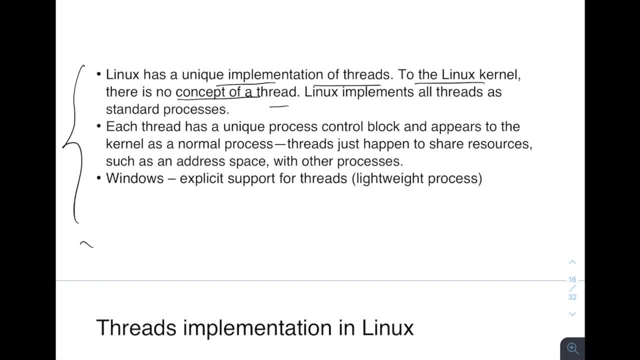 linux does not differentiate much between process and the thread, so linux, what it does, is linux implements all threads as a standard process. i will show you how it is done. each thread has a unique process control block. so a process has a process control block and a process control block. 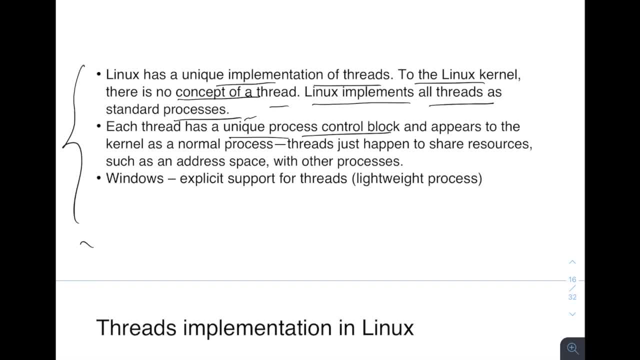 thread also has a process control block in linux, i am telling, in windows it may be different, and to the kernel it appears as a normal process itself, only difference being that threads just happen to share resources, which process do. not only this is the difference that linux sees in threads and 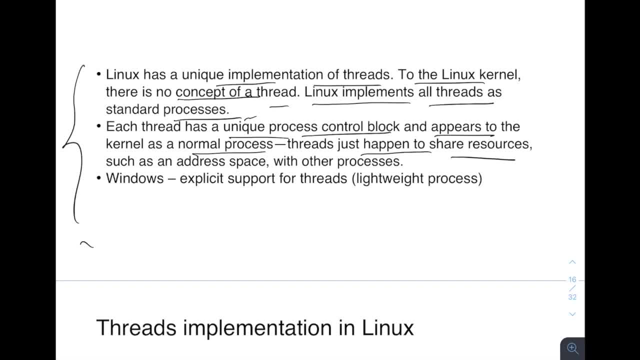 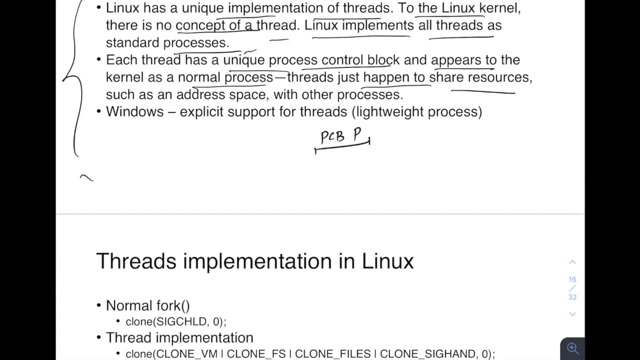 process, nothing else. they- i mean threads- also has process control block. process also has process control block, only difference you. you understood this right, only difference that. so okay, understood. so let's say: this is the pcb for a process, for a process, p process control block. in that 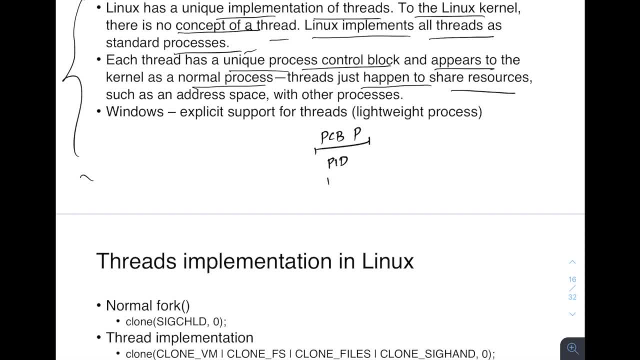 different information like pid registers. i will say stack memory, heap memory, data memory, a code segment memory. these all are stored in pcb pop process. let's say you have pcb of thread, this also. you have pid registers, stack heap, data code. the difference here is that if let's say process, i mean of course. 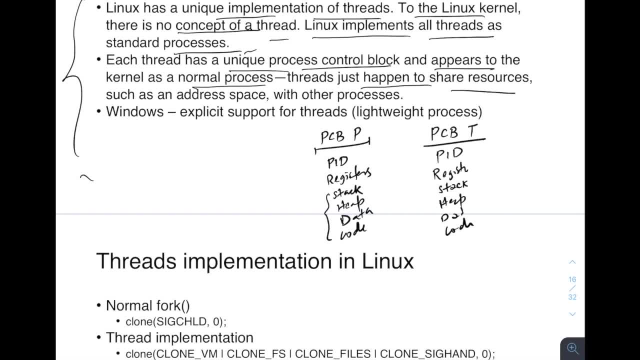 thread are not independent. they are created within a process itself. let's say that trade was created in this process p, then what will happen is this: this, i mean these four parts, will not be duplicated for this thread. so this stack pointer let's: this is the pointer. this will just point to this stack. 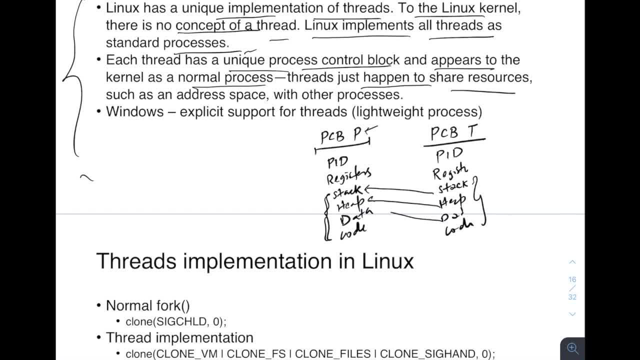 i mean this pointer, this will just point to this. this will just point to this, this will just point to this. so this all will basically share the uh sorry, sorry stack will be different. sorry, a stack should not point. stacks will be unique for both, but all the other three sections of memory it will. 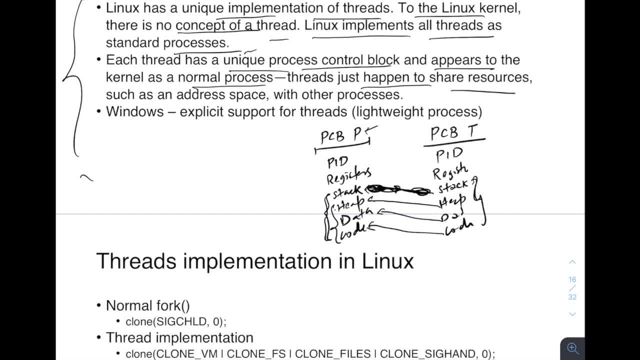 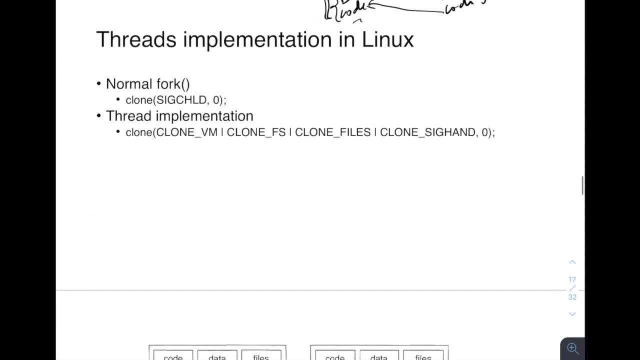 just move point, i mean use a pointer to point to this. they will not make a duplicate of this heap memory, data memory and uh code memory. so that's the how linux implements this, right, it's quite easy for linux, right? they will just use a pointer to point to it, quite it becomes quite easy. see this, uh like. 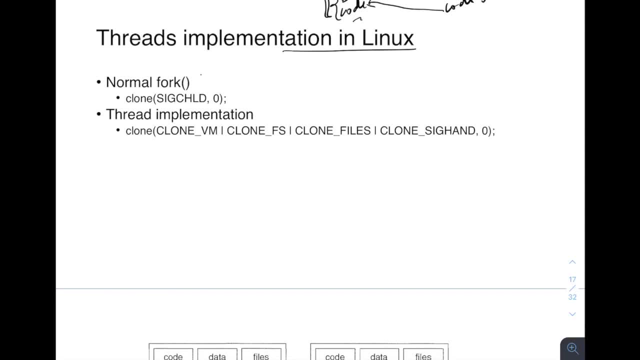 how threads implementation happens in linux. so when you are using uh, so fork is used for process creation. when you use a fork, you can create multiple process. now, in this, what linux does, is it? it normally uses this clone system, call so clone. so actually i will say that uh. in previous 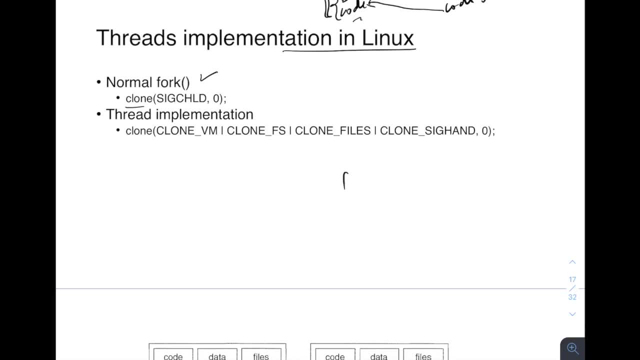 linux uh version versions. uh, fork used to be a system call, but today linux is using a system call. so in previous linux versions uh fork used to be a system call, but today linux is using a system call. but today, now it's not so. fork is just a, i will say api. uh, that is a library itself and clone is the system. 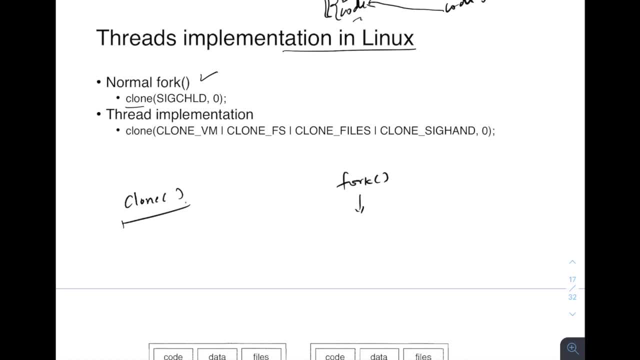 call for creating process or trade. so using this clone system call the, linux can differentiate between whether you are creating a process or whether you are creating a thread. so if you see here in this you are just sending the uh, sick child signal. so that is like a parent normally. 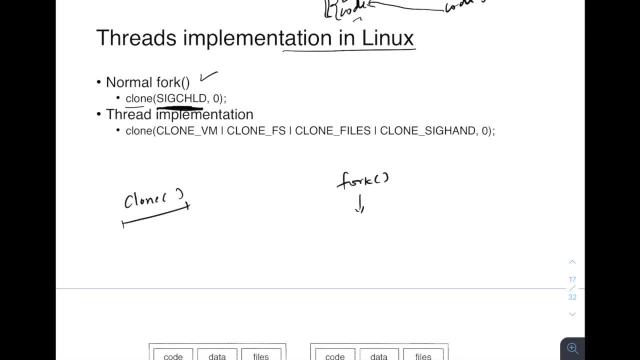 waits for uh its child, right, and some signal will be sent when the uh signal is sent to the child, when the child process is killed. so do not go into advance of this. i'm just telling that if you see the parameter passed here for creating process, it's just this one parameter. see the parameter. 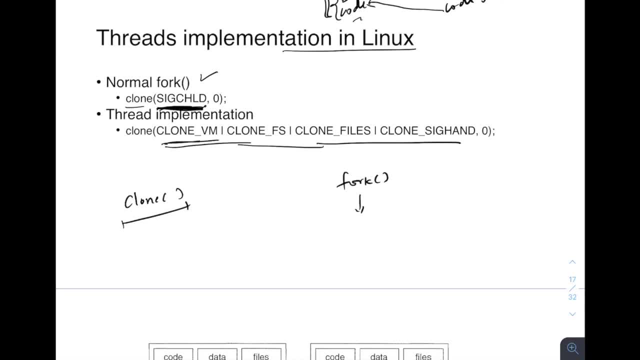 passed for creating a thread, right. you are passing like: clone the virtual memory, clone the files, clone the signals, right? so that's what how the linux different differentiates: when you use this system call, thread is created. when you use, i mean, system call is same, but when you use these parameters. 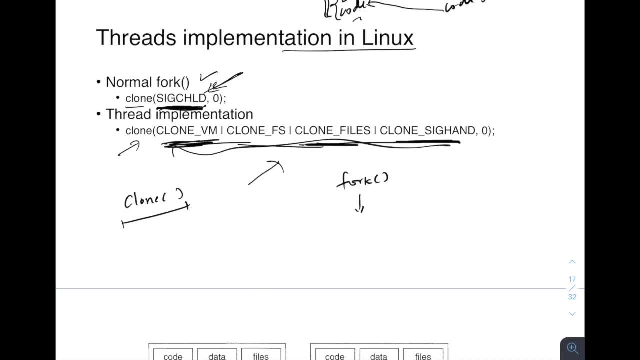 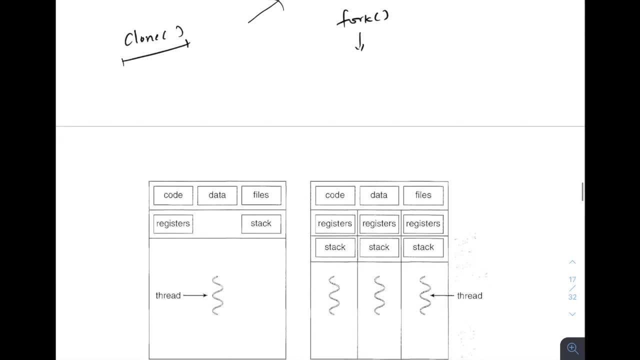 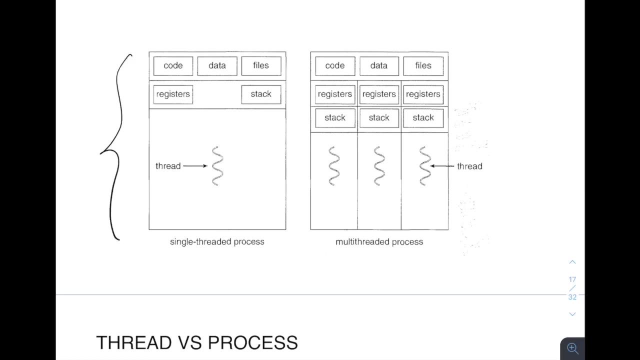 of course process is created when you use these parameters. you get a thread. so of course, thread, if you see, the parameters passed are so that they can share the memory and files. this is another diagram to show the difference. if you see, this is a single threaded program. so see, even if, uh, if you, even if you have a process does not have like multiple. 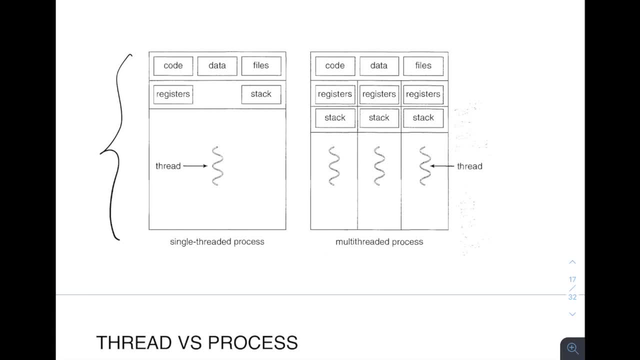 threads. in that case also you have a single thread of execution, because thread is mostly concerned with this thing. right, code, data, uh, mostly code and registers and stack. right, that is a thread. so every process has a single thread of execution. but in case you have, if you have multiple threads, 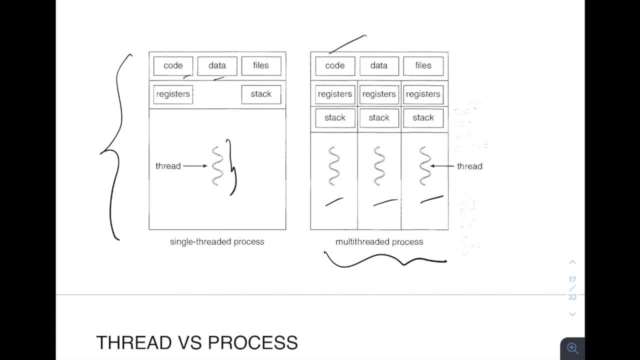 like three threads here. if you see, here each of this is sharing these three, right, all are sharing this code, data and files, but for each of this, the registers and the stack registers and stack register and stack are different, right, that's how this happens between the difference between 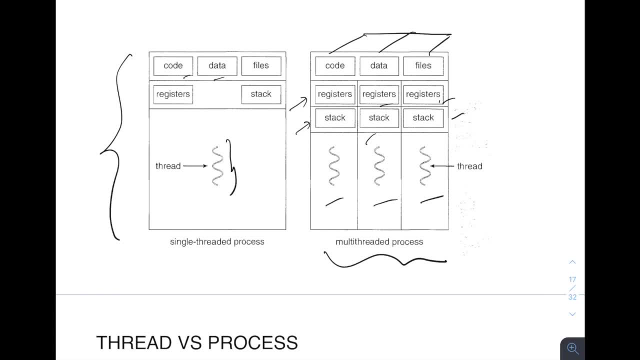 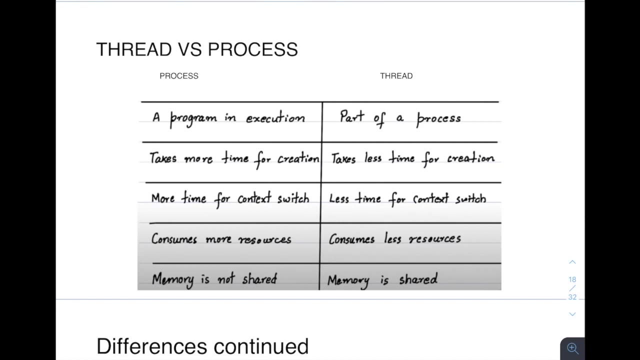 process and thread. in process, everything will be duplicated in threads. only i mean i will say: all will save these three things and this all will be created new for them. okay, i have already discussed the difference with process and thread, but let's revise here. a process is a program in execution. thread is, of course, a part of a process itself. 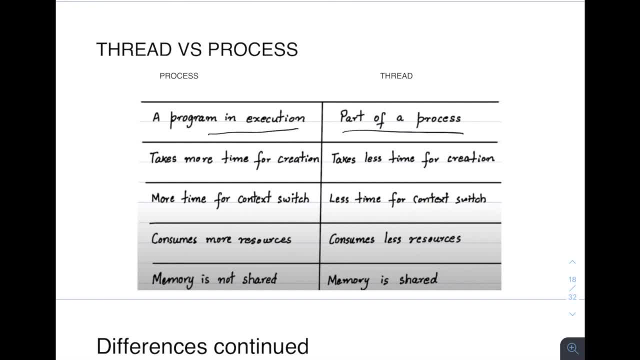 it's not a different- i mean independent- entity, it's a part of process itself. you cannot create a thread without the process. first you create a process, then you can create multiple threads within that. process takes more time for creation, of course it will take more time because you have to reduplicate all the memory. 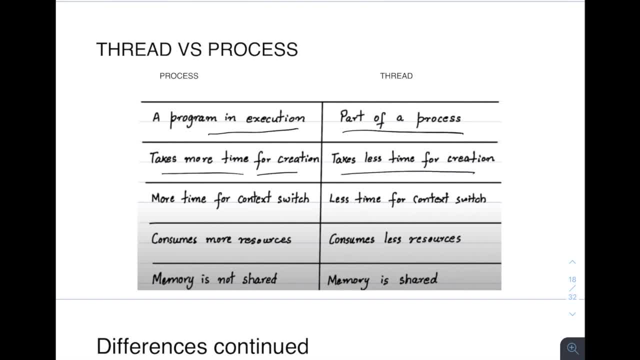 here. you do not have to really duplicate all the memory. you only have to create a separate stack memory. other three segments of memory remain same. more time for context switch here. less time for context switch here. this is because, uh, so this is related to memory management. so what happens? 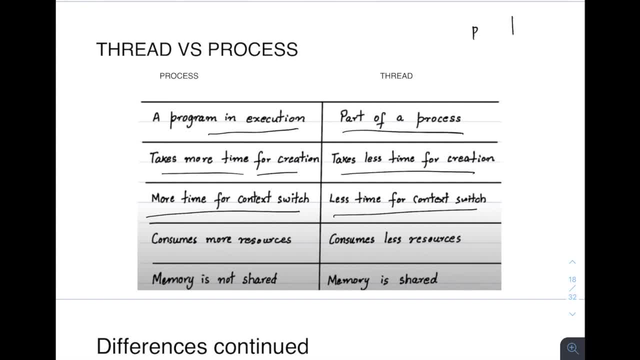 every process, every process p has a page table associated with it. so this page table actually uh helps in converting logical address into physical address. now, uh, see what happens, see what will happen, and also in context, which what happens. you have normally cpu here. there are a lot of registers. 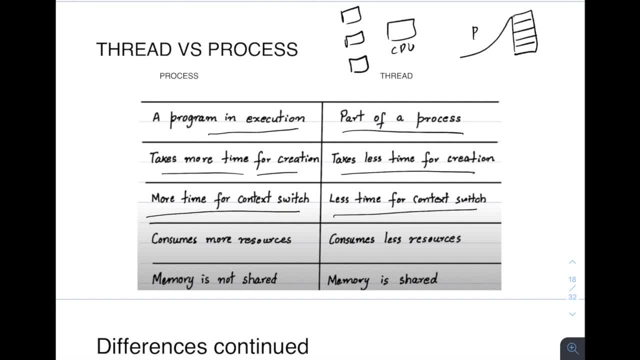 and in one of the registers the base address of this page table is stored. so every process has a unique page table. so of course, the base address will be unique and their base address is used to store in the registers. now, when context which switch is happening, this, i mean this value, i mean the value in these registers needs to be changed. i mean when the 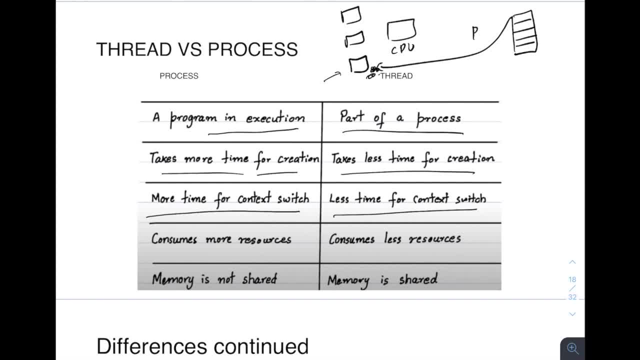 context, which is happening in different process. why? because each process has a separate page table. of course, you need to replace this register with the base register of the new page table, right? but think in terms of threads. in threads, each thread is sharing this page table, right? each? 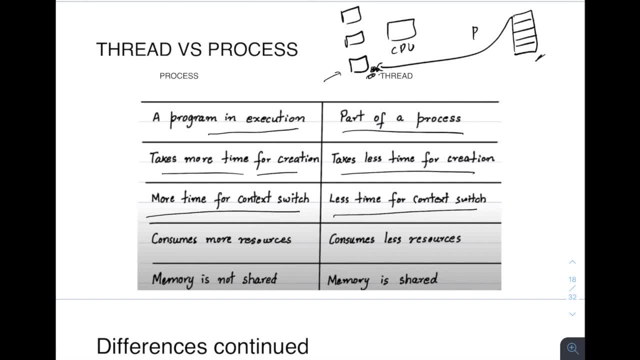 thread does not have different page table. all are sharing this page table because this page table is mapping and the memory mapping for all the threads are same. i mean all the threads within a process are same for them. this and when threads are context switching, when i mean threads within. 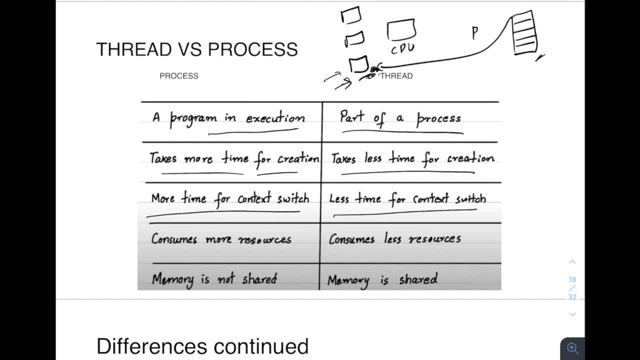 the same process are context switching. the kernel does not need to change this register value, the base register value. that's why i told i mean this. context switch time of course consumes more resources. when you are reduplicating the memory, it will consume more resource, more memory. this. 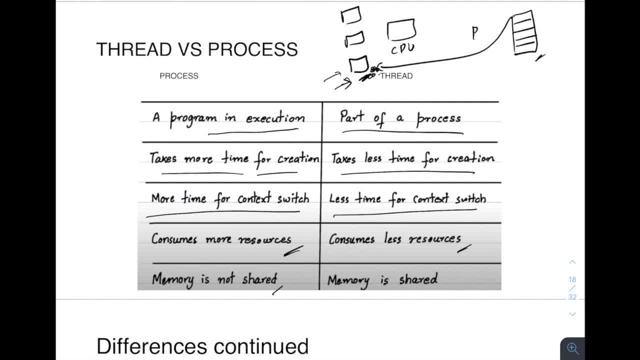 consumes less resource and this is a basic difference that makes all the difference. actually, memory is not shared here. memory is shared, so only stack memory is different for process and thread. uh, i'm sorry for multiple threads. if you have multiple threads within a process, the stack memory for all the threads will be different, but other three segments of memory will be same. 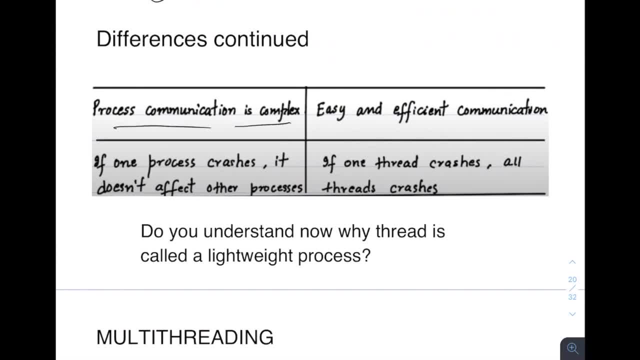 now let's continue the differences. uh, process communication is complex but it's easy and efficient. uh, for, like, when you have threads, of course, in threads it's quite easy, right, you create a shared space and write and read to it, right, quite easy. process communication can be tough, like when you want. 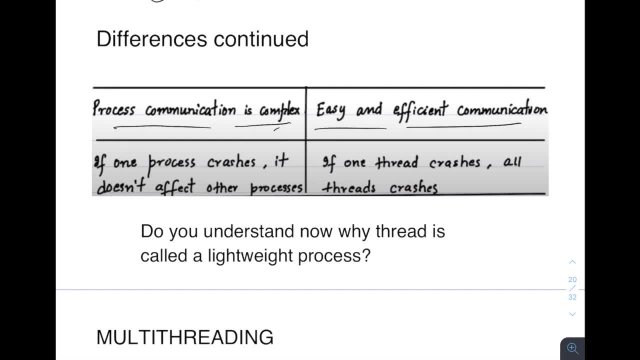 to write: uh, use like soccer programming, or uh, maybe rpc or pipes. it can become tough, and in the program code itself can be quite, because there are system calls here. so it can become quite tough, but thread programming is quite easy. i will say than this the one disadvantage with threads: 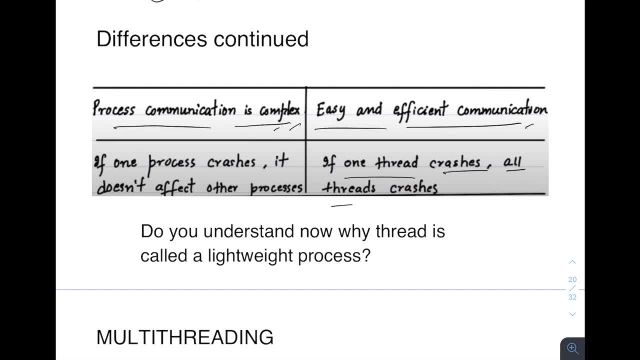 is that, uh, if one thread crashes, all the other states will also crash. this is a disadvantage with threads for a process: it does not affect the other process. if one process crash, it does not affect the other process. and this is. i will talk about this when i talk about chrome and firefox, at last. 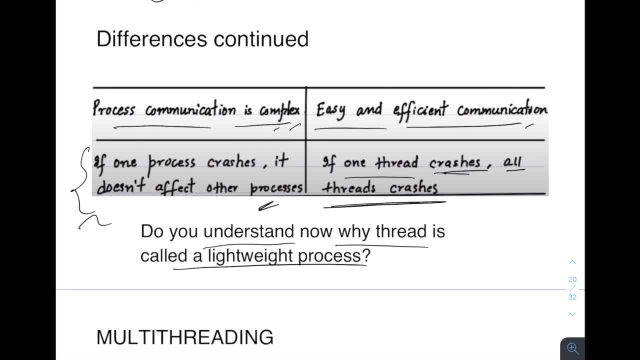 now, do you understand why a thread is called a lightweight process? do you understand this? if somebody asks you why a thread is called a lightweight process, so you understand it's a lightweight in the sense that if your thread is sharing a lot of resources with other threads, that's. 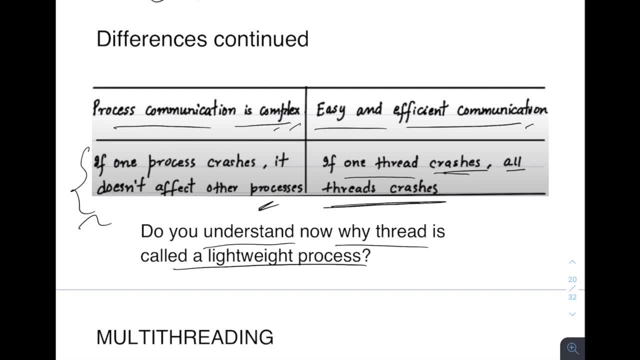 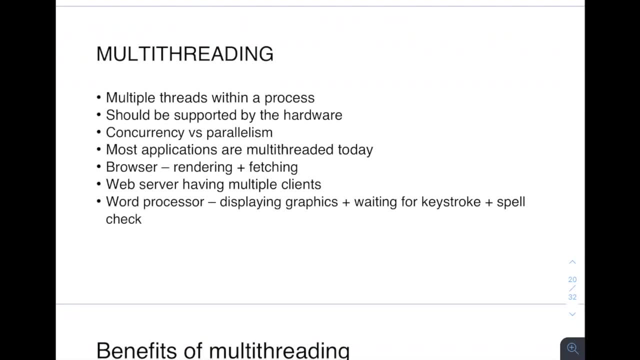 why it's light. a process is re-duplicating a lot of resources. that's why it's heavy. understand this difference. okay, now you've understood. uh, what is thread difference in process thread? the famous interview question. let's now move to multi-threading and multi-processing. of course, multi-threading is. 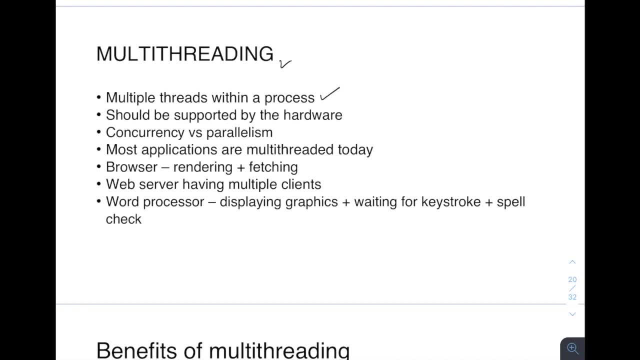 when you are using multiple threads within the process. so you, when you have multiple threads within a process, it's multi-threading, quite simple. so multi plus threading, multi-threading- it should be also supported by hardware. see, if you have only uh, one cpu, or i will say one core, and i mean if, even if you write a multi-threaded program, 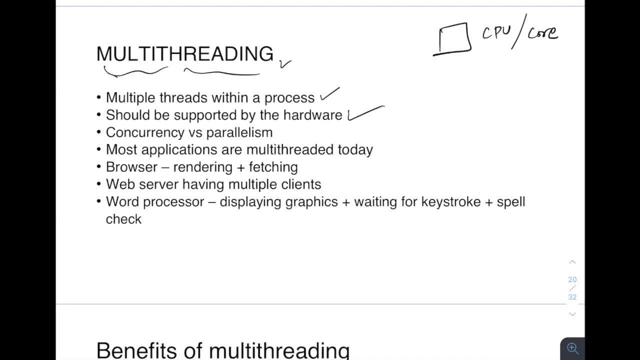 it's of no use because it your, your hardware only supports a single thread. even if you write a multi-threaded program, it will not make it faster. understand this, so that's why hardware support is needed. and also understand the difference between concurrency and parallelism. both are different, so you will think that both are same, but both are not so concurrency. 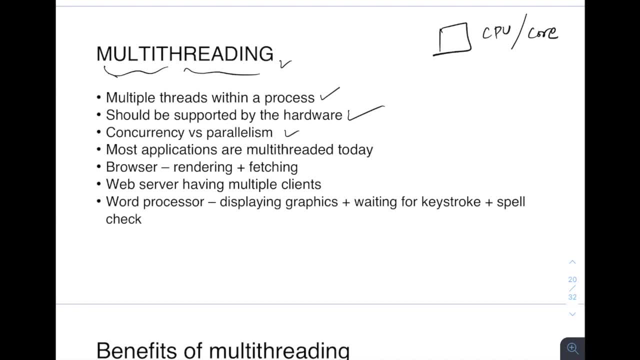 is like: okay, concurrency is kind of i will say, uh, it's almost parallel, but not actually parallel. okay, so the differences, so concurrency is something like this. so this is your cpu highlights. sorry, you have one cpu here and let's say the cpu. this is the time interval on which 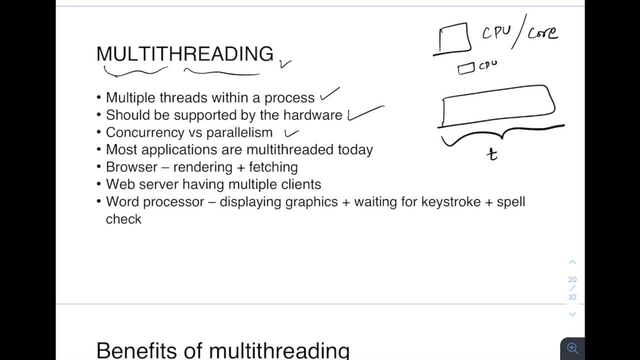 the cpu will run. let's say this is the time interval. now some process will keep on arriving. so the cpu, what it will do is it will give some time to p1, next to p2, P3, P4, again P1. So this round robin fashion. So basically, this is the role of kernel itself. 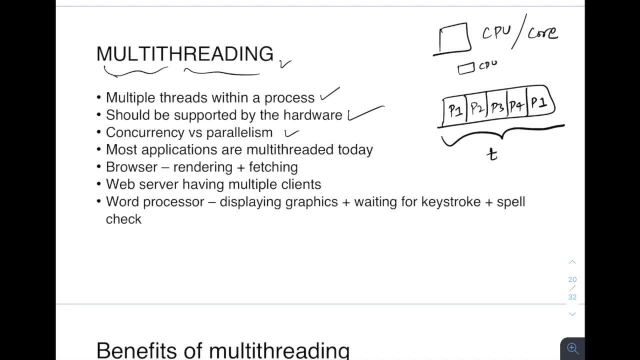 The kernel will use round robin scheduling algorithm and this will keep on happening. So this is concurrency. Why? Because every process is getting some slice of CPU time, Let's say 10 milliseconds. To the user. it looks like it's parallel because it's happening very fast. 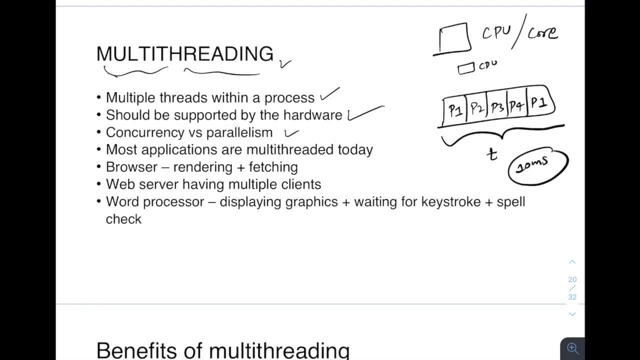 Like they are maybe browsing. they are typing on the text editor. Everything is happening very fast. So to the user it looks concurrent. right, It's almost concurrent it looks like. But this is how it is implemented here. But parallelism is different. Parallelism will be faster than 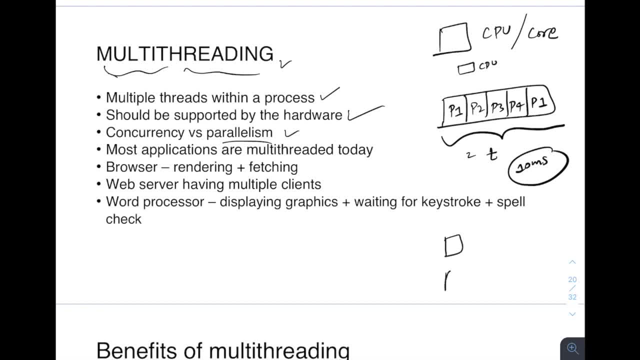 concurrency. So in parallelism, what happens? You have multiple CPU, So P1 will be running on this CPU, P2 will be running on this CPU, P3 will be running on this CPU, And this will be very fast. 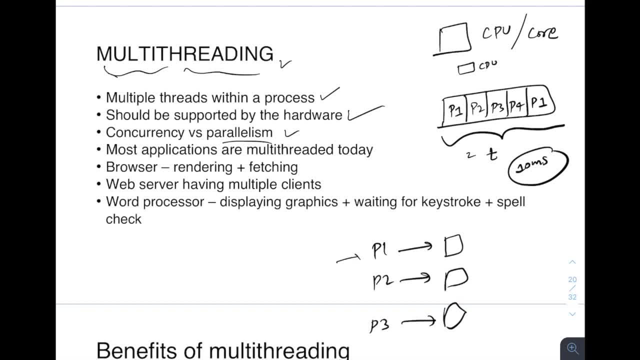 because P1.. So in this there was context which was happening right Between process. But this context, this was happening very fast Here. it's not so Each one is running on this CPU And this will be very fast because P1.. So in this there was context which 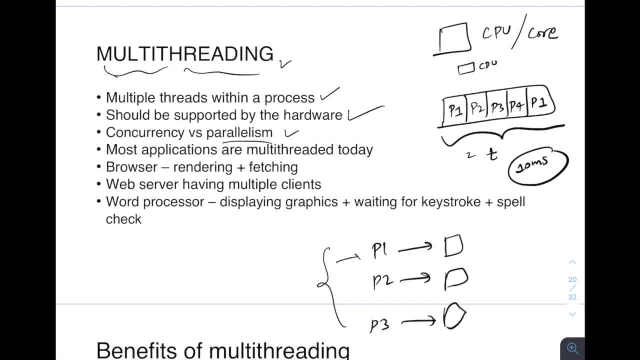 is running on a separate- I mean CPU itself, So this will be very fast. So this is called parallelism and this is called concurrency. And concurrency can happen also on single CPU itself. right, That's what I showed you. But parallelism cannot happen on single CPU, You need multiple. 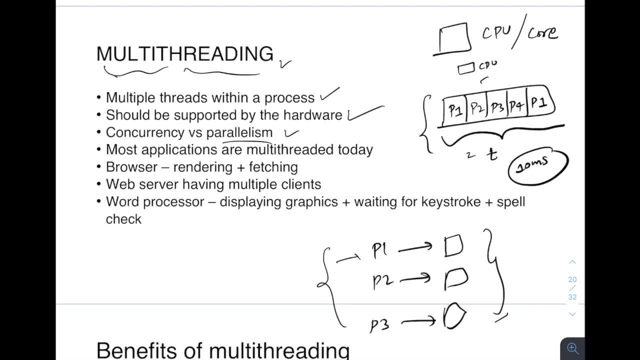 CPUs, for I mean parallel programming. Also, most applications are multithreaded today, Like most of the applications you see on your desktop or laptop. Your browser is multithreaded. Your web servers? You do not have a web server, But let's say Amazon, Google, they have a lot of web. 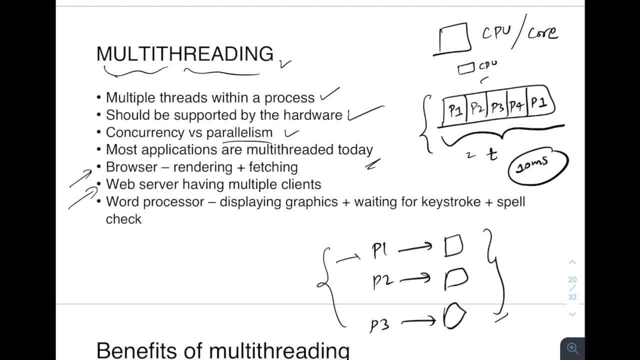 servers And all the web servers are multithreaded. Even word processor that you have or text editor that you have, they are multithreaded. So browser is multithreaded in the sense that a browser does a lot of stuff. It renders the content of the HTML on your browser. At the same time it also has to 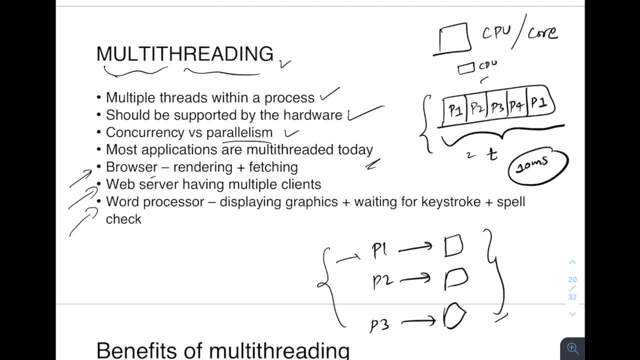 face this information from the web servers, So it will use a multithread to make this faster. Similarly, web servers like see Google will be handling like requests from you, from your friends, from everyone from your family and a lot of users globally right. So it has to make this very fast, So it will use multithread. 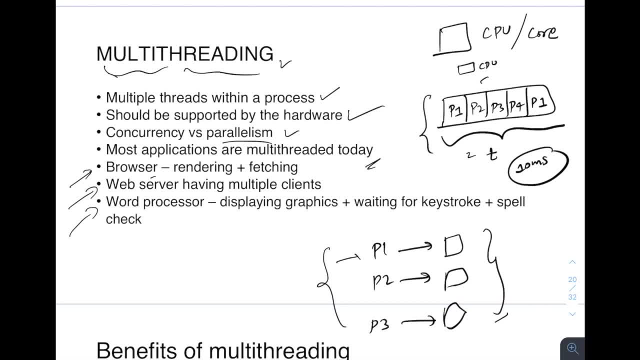 and handle all these connections separately. Similarly, word processor- if you see it is also displaying you graphics. It is also waiting for your keystroke right. It is waiting for you to type. When you type, it is also doing spell checking. So there are a lot of functions it is. 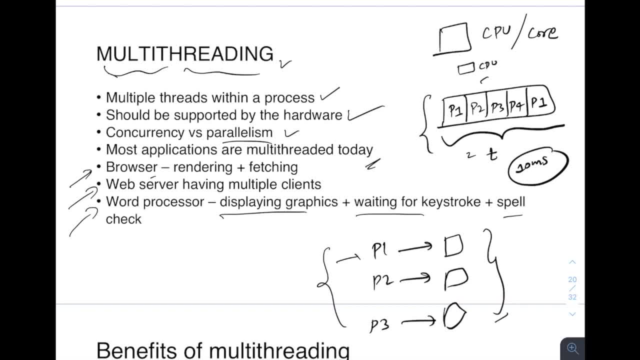 doing one single thread, then this will be sequential and it can be slow. To make it fast, what it will do is it will use multiple threads. One thread will help in displaying graphics, One thread will help in waiting for keystroke, Other thread will help in a spell checking. That is how it can make fast. 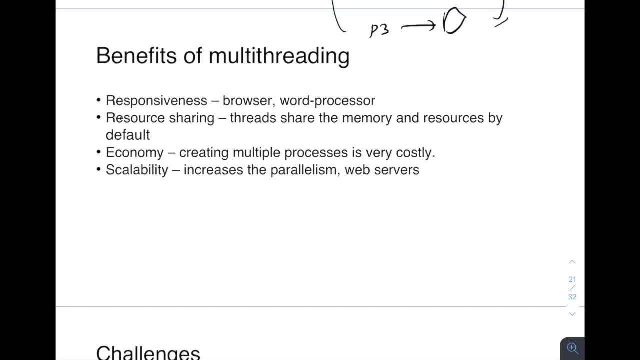 Of course. but now you understand benefits of multithreading. Of course responsiveness is one of the. I mean you think of a browser and word processor. I mean, Let's say, if you are not using multi-threading, the time of the browser or word processor will be slow, because browser will first. maybe. 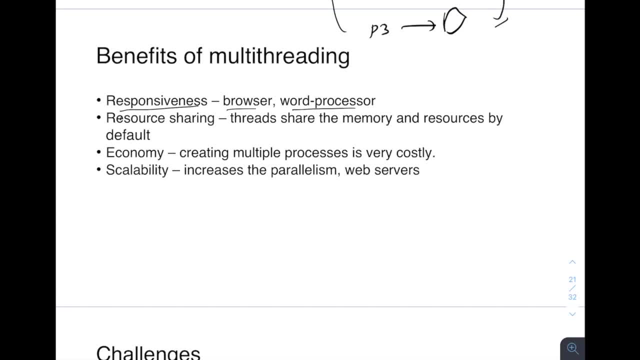 phase the information. after phasing the information, it will start rendering. and also, if you open another tab and open some other site, it will be sequential and it will take a lot of time. Similarly, word processor: the spell checking can be slow if it is running on a single thread. 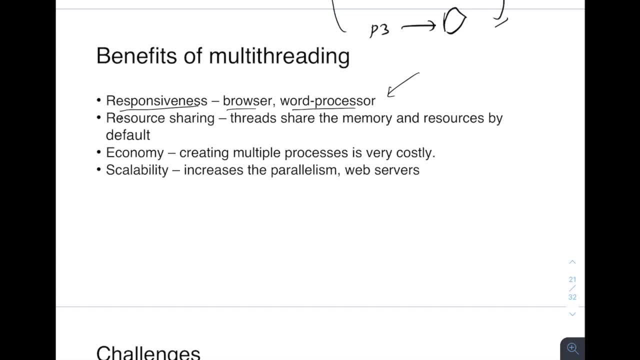 When you are typing, normally spell checking is very fast, but now when you are typing after you type, it will do the spell check, so it can be slow. Of course, benefits of multi-threading is resource sharing, like thread share, memory and resources by default, so of course resource sharing is there. 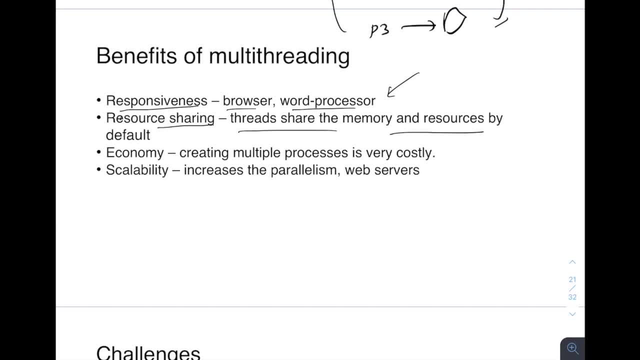 Other is economy. is there economy in the sense that when you are creating multiple process, they are costly, in the sense that you are duplicating a lot of resources? In multi-threading it is not so. in multi-threading you are not duplicating a lot of memory. you. 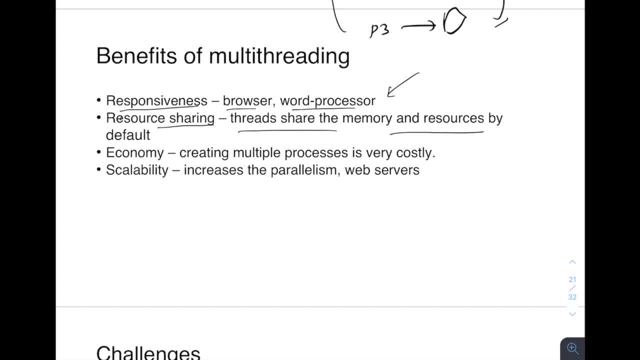 are sharing those. that's why it is economical. But of course, last one is scalability. it increases the parallelism. like I have given the example of web servers how they can handle a lot of clients using multi-threading, So these web servers can scale a lot in this sense. 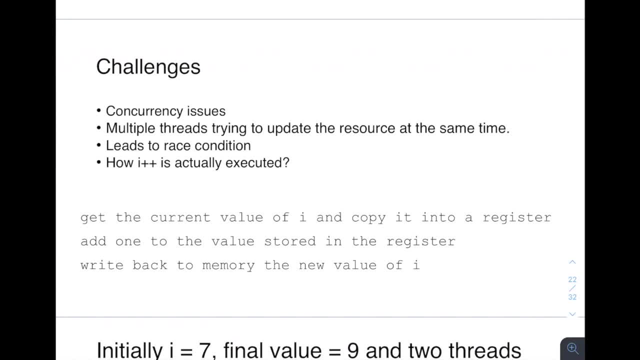 I also understand what are the challenges of multi-threading. this is also very important, like what are the challenges for multi-threading. So multi-threading is very- I mean- good concept. it is very fast. there are lot of advantages of it, but there are some challenges here also. 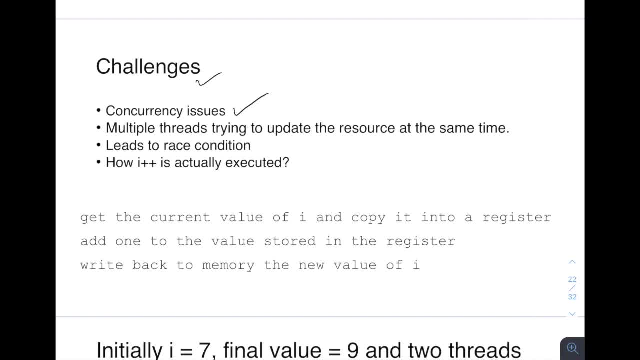 There are concurrency issues that can happen. I will show you that with the example. like this will happen, like when multiple threads trying to update the same resource at the same time. at that time it will lead to raise condition. So I will explain this with an example. it will become very clear. 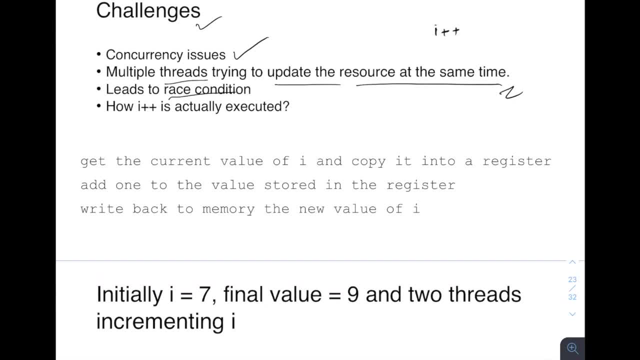 So think of this: when you write I++ in your code, let's say so, what happens? what do you think? so, actually, of course, this instruction gets converted into machine level code and then the CPU will execute this. But what are the instructions involved here? 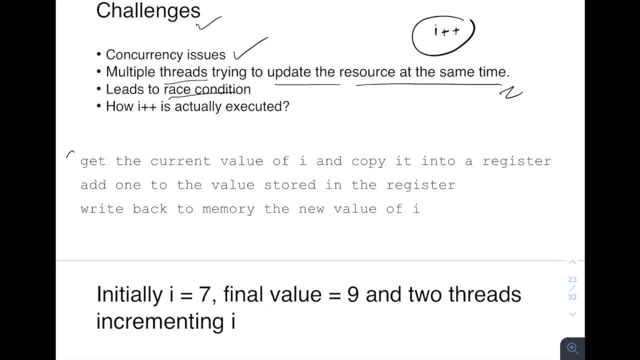 So I++ is actually a combination of three instructions. I have not written the instruction name here, but I have written what those instructions actually do. So the first instruction will get the current value of I from the main memory and copy it into a register, because CPU has to execute this instruction. 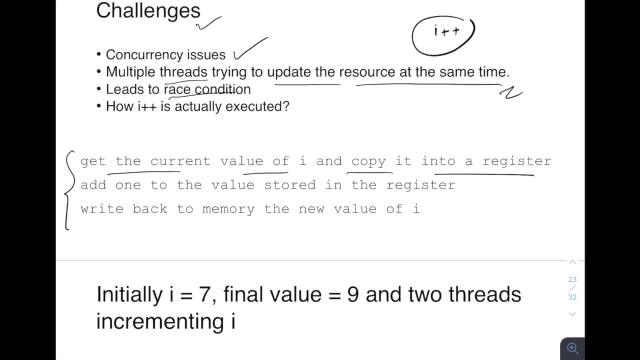 So that's why the data first has to be phased from the RAM to the register. After this, the CPU will add 1 to the value stored in this register. So the CPU has ALU with it. this ALU- I am automating a logical unit. this will help. 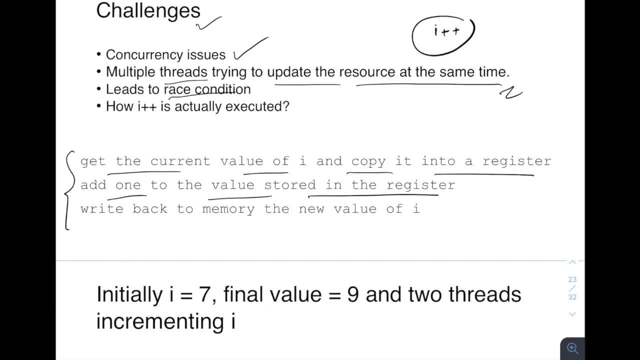 in adding 1 to this value, whatever initial value of I is, and then again it will be stored in the register, But finally the CPU will write back this updated value to the main memory. These are the three instructions involved. Let me show this with an example, like when you take an example of, let's say, your initial 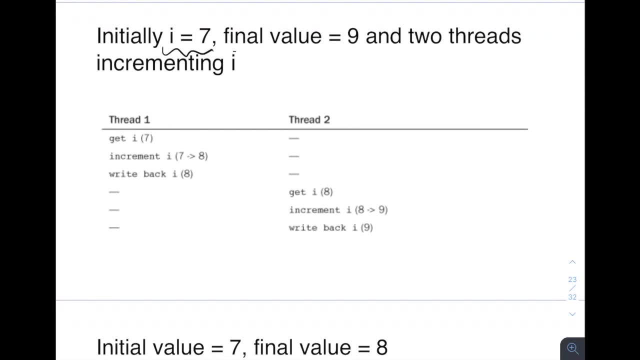 value of I is 7, let's leave the final value and you have two threads which are trying to increment. I So think about this. when you create two threads, both can. so let's say this is a function. maybe you have a function increment. this is a function increment. you have a global. 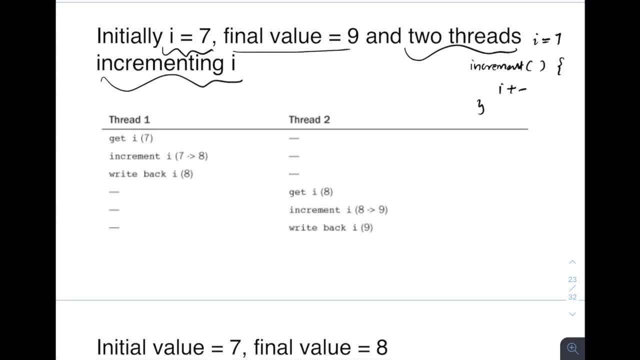 variable I, the value is 7, in this function you are doing just I++. Then you have, let's say, main function. in this you are creating two threads, T1 and T2.. Then you are doing, let's say, T1- start. I am just writing a pseudo code here. it's not. 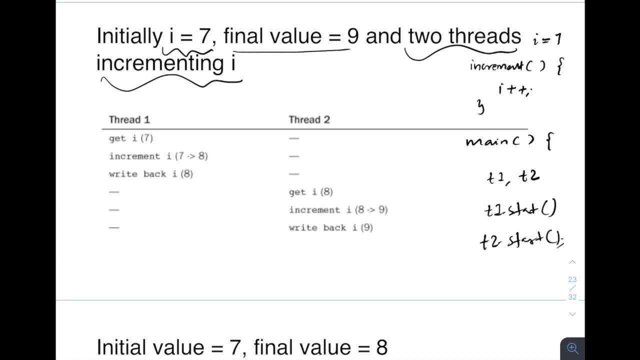 actual code: T2- start. let's say you are starting both the threads or running both the threads. Now you do not know both can actually start executing this function at the same time. this can also happen. I mean, you do not know about the order whether both can start at the same time, or it may. 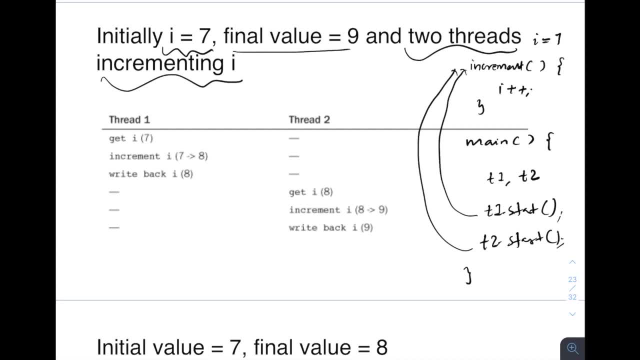 happen that Because T1 executes, then T2, or opposite can also happen. it all depends on the your, the kernel scheduler, how it schedules it, because both has started now it depends on kernel when it schedules this, So that's why concurrency issues can arrive. 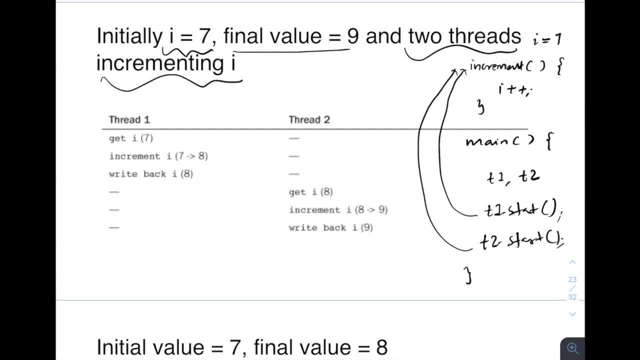 Now I will show you what issues can arrive here. See this: okay, now this code is there, so you will basically run this program. So, of course, this is your. let's say: this is your, this is your RAM, this is your RAM. 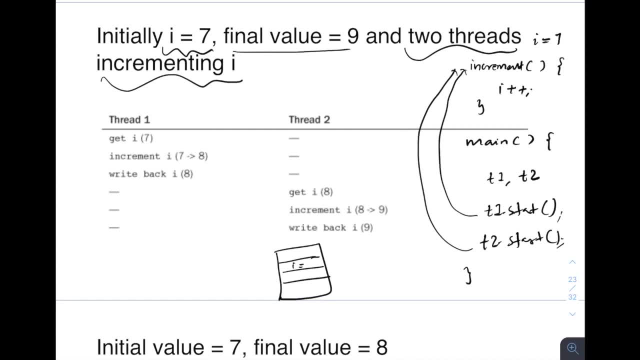 this program is loaded in the RAM. I is 7,. let's say it is stored at this memory address. let's say, Now you have CPU here, it will have registers. So okay, let's say this is the time T1,. I will divide this. this is the time T2, this 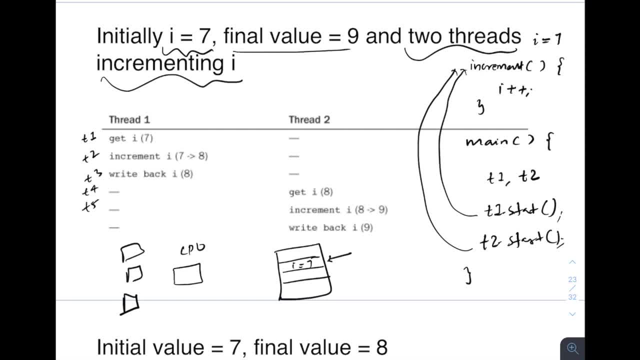 is T3, this is T4, T5, T6, I have divided this into timeline. so T1, of course, is lesser than T2.. T2 is lesser than T3.. This is your timeline. Now let's say this is the sequence. 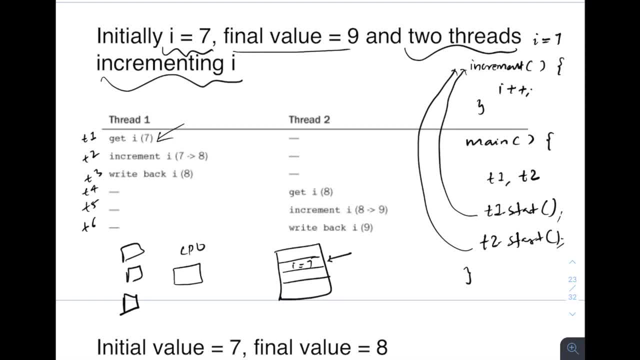 So first, at time T1, thread 1 gets the value of 7, that it gets the I value to the. it basically copies the value of I from RAM to some register. Let's say this is the register. here it's copied. 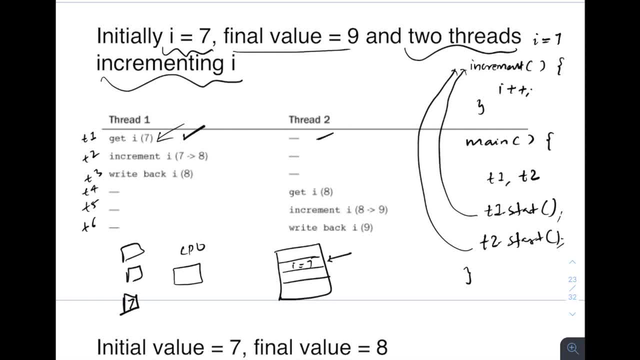 First step is done. Thread 2 does not do anything at that time. Next is increment I to 8.. This will CPU will do right, using the ALU. it will increment this to 8, let's say it has incremented. 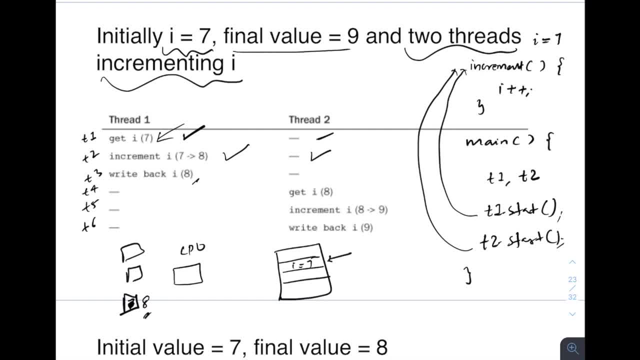 Again. thread 2 didn't do anything. here Again, last step is write back this I to the main memory, So this will be written to here. from 7, the final value became, let's say, 8.. That's good. Now, after T3, at T4,. this has finished. the I++ has finished. 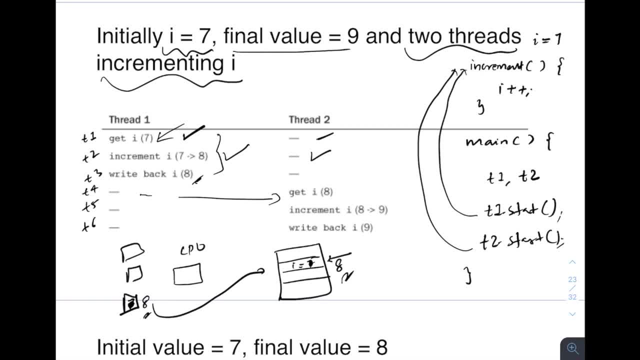 Now at this thread 2 actually starts executing the I++, So it will get the value 8.. So okay, let's say same CPU is executing this, So let's say it will get the value from here, let's say in different register here. 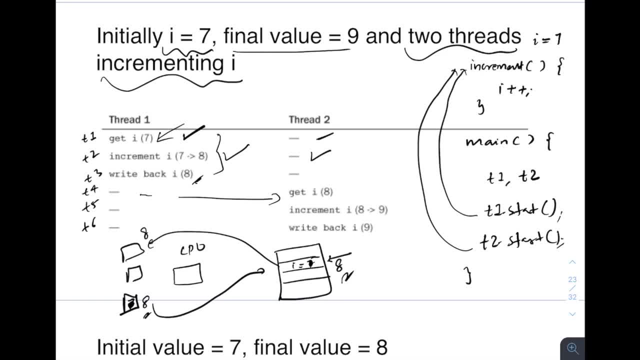 I'm just using, So make it clear, I'm using different register. Then it will increment to 9.. So it will do to 9.. And then it will write back this. So it will write back update. it will update this to 9.. 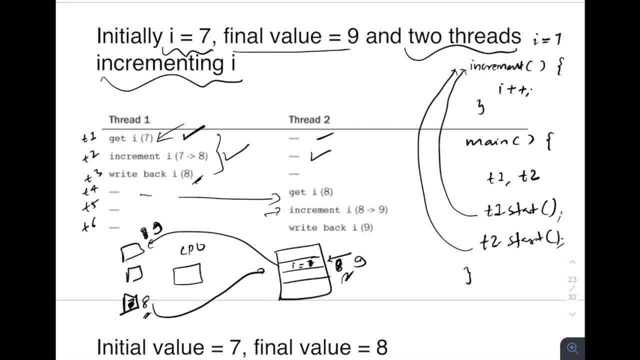 So this will happen right, Everything is good here. The final value got 9, two threads were there. initial value was 7.. So last value should be 9.. That's quite good, Everything is good. Now understand this one. 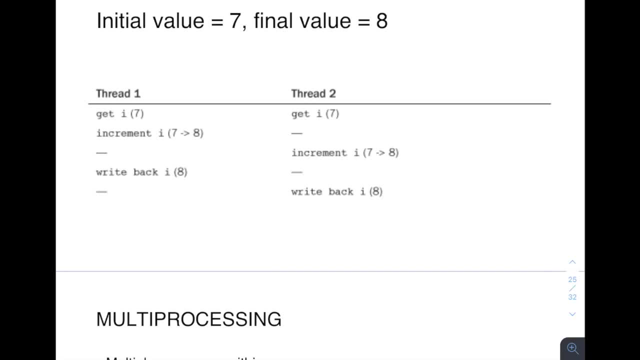 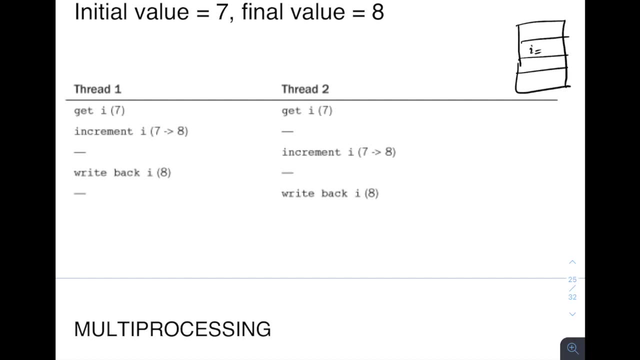 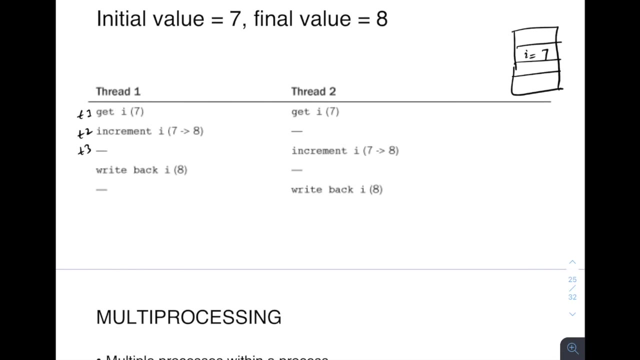 In this case, the issues can happen. Understand this very clearly. Again, you have RAM here. Let's see, You have started running the program. initially, I is 7.. Now again, divide this, sorry, divide this into T1,, T2,, T3,, T4,, T5, okay, there are only. 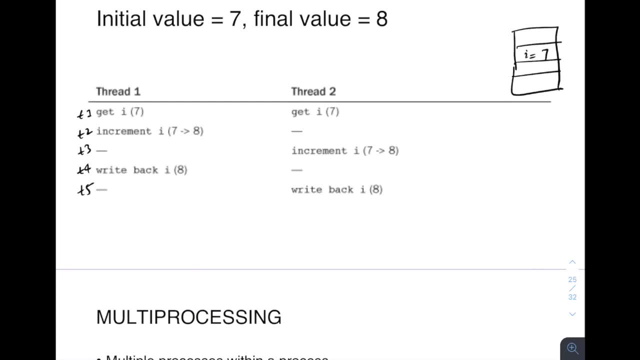 T5. here let's say: And let's say, okay, we will take two CPUs. here Let's say: this is CPU for thread 2, it has registers, three registers, So CPU for 2., 2., 3.. 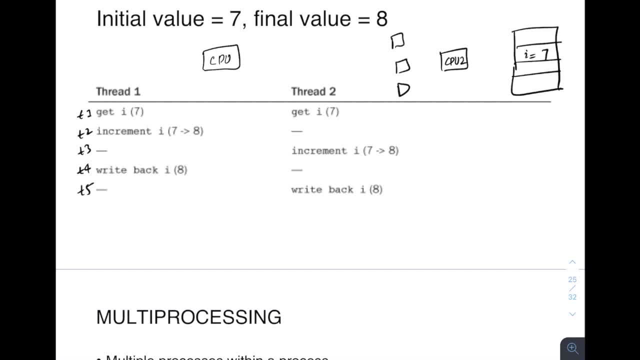 4., 5., 6., 7., 8., 9., 10., 11., 11., 12., 13., 14., 15., 16., 17., 18. 19.. 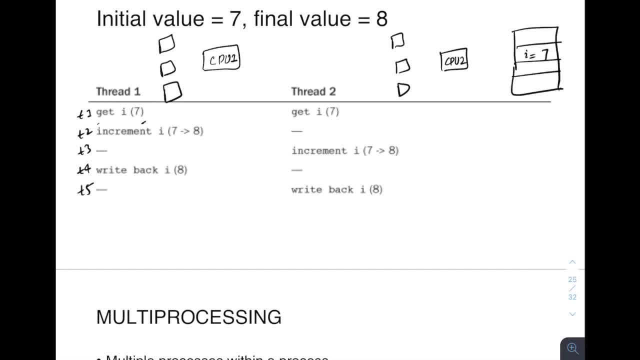 21., 22., 23., 24., 25., 26., 27., 28., 29., 32., 33., 34. for thread one cpu. now this gets into this register. both have got the value from main memory. 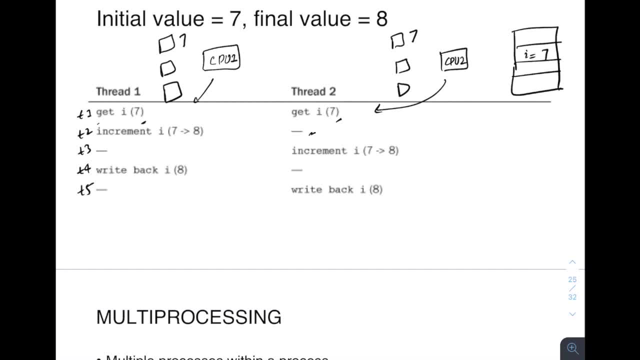 now at time t2, uh, for this nothing happens because maybe, uh, this was maybe removed from that cpu it context, which can happen, because that all depends on the pause scheduler for this. what happened? it was still running and it incremented this to eight. now at t3, uh, this maybe got context switch this. 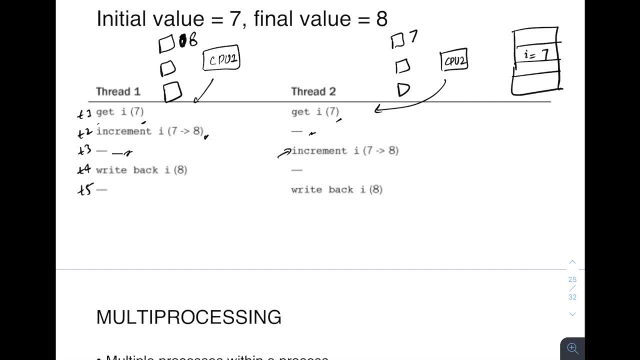 process. thread one got context switch and this uh increased this to eight. all good at t4. uh, what happens? this is writing back the thread one is writing back eight to eight to here, so it will write here. i mean it will update here from seven to eight. i value, and three, two didn't do anything. 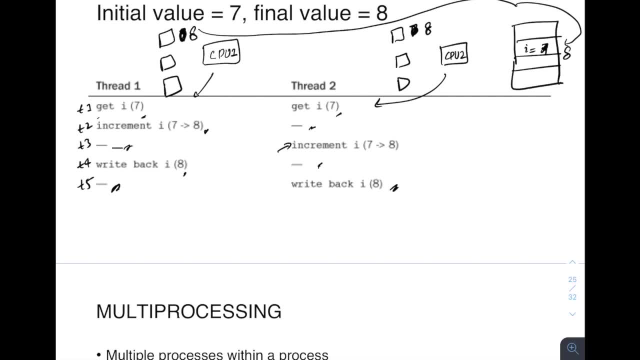 at t5. of course this is completed. this will not do anything. but this is again writing back the value of eight to the main memory. so it is will also write, update it here and overwrite eight to again eight, same value. so if you see here what happened, the final value was eight, it's not nine. that's why i told concurrency issues can. 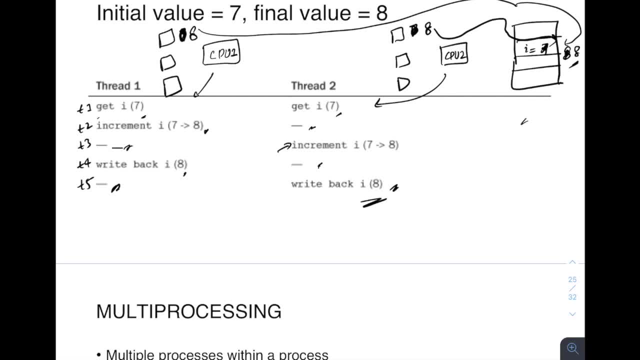 happen in this case. right, so that's the issue. you will expecting the output to be nine, because two threads were there, but output is actually eight. and if you see, what is actually happening is that, since this consists of three instructions, i mean both are clashing somewhere. right, in that that? 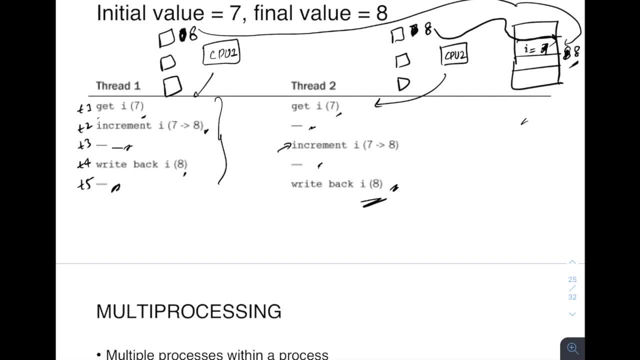 case it's happening and that's this is called a race condition, because both the threads are racing to update this value. that's why it's race condition and this can cause issue. this is very dangerous. actually. the race condition and also identifying this is very tough. we'll discuss the solution to this in process synchronization chapter when we cover that. 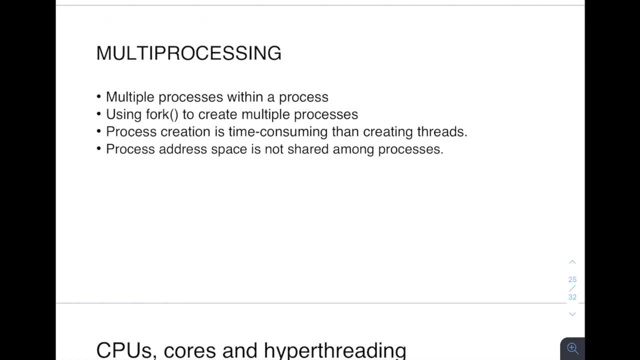 okay, this was about like: what are the challenges to multi-threading? let's now move to last part: multi-processing. so of course multiple processes within a process is multi-processing. you use fork to process multiple processes. of course process cost, occasionally time consuming, that creating threads i've already discussed. and of course process address space is not shared among. 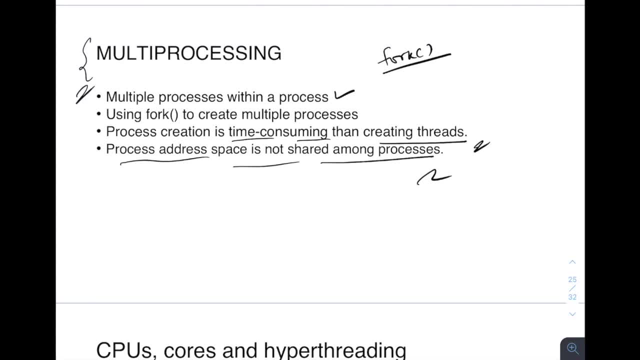 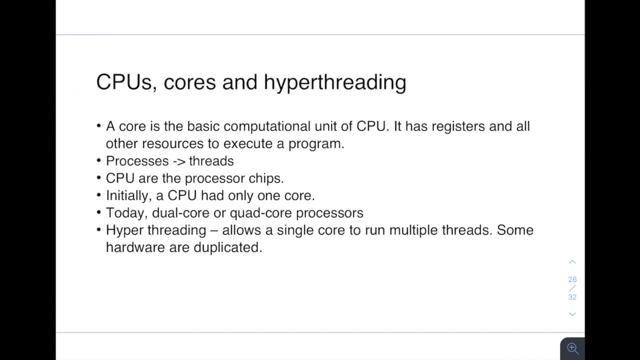 multiple process. so of course multi-processing will be normally slow because of this. let's also understand about cpu codes and hyper threading. so a core is basic computational unit of cpu. so cpu is normally like you have a hardware chip on this left. there can be a lot of cores. 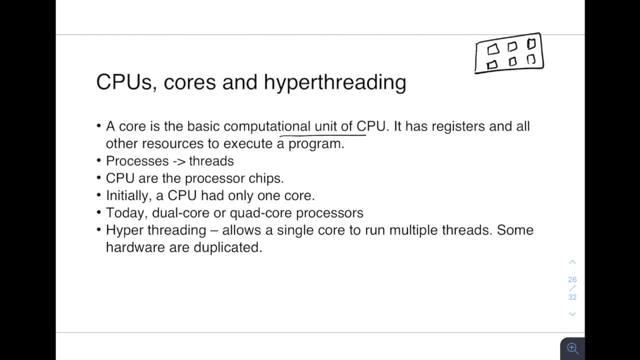 now, each core is the basic- uh, i mean unit of CPU. Each of these cores will have registers and ALU, and all This also will have different registers. So each of these cores has registers. So this is basically a core and this whole thing is basically your processor chip or CPU chip. So, similarly, in 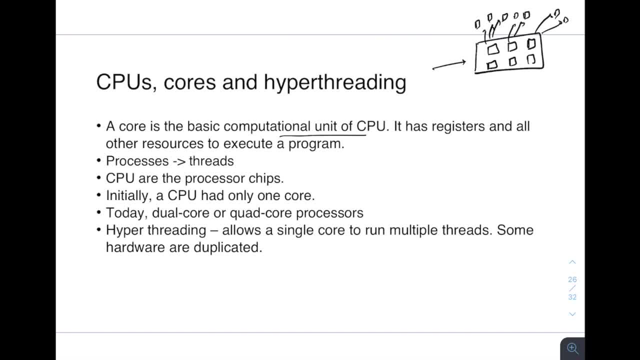 the case of process, you have processes Within processes. you have multiple threads. Here also you have a hardware chip like CPU chip or processor chip. Within a chip you have a lot of cores. So, okay, this I have explained. Initially a CPU had only one core, I mean. 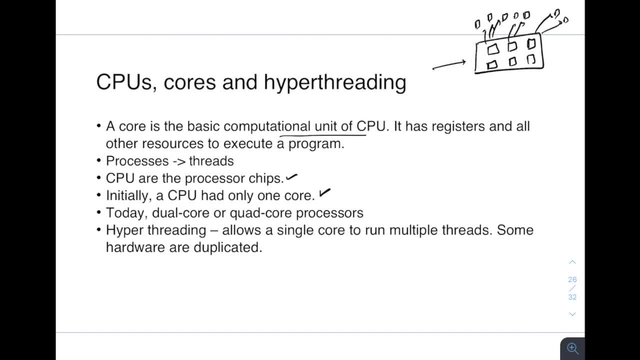 in old times you had like CPU with only one core, But today you have dual core or quad core. Dual core means you have two core processor. Quad core means you have four cores. So in modern, of course, in modern operating system, we will have dual core or quad core Then. 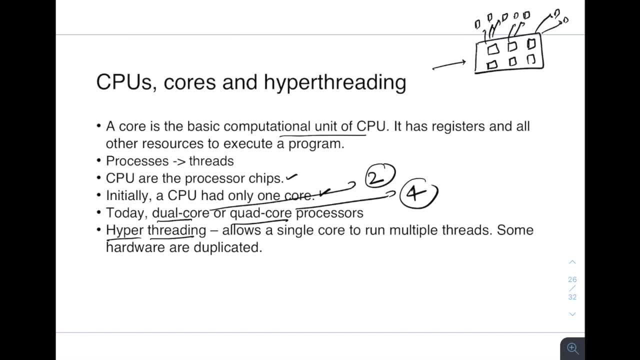 you have again another functionality called hyperthreading. So if hyperthreading- you know, if hyperthreading- is enabled on your hardware, what will happen? It will allow a single core to run two threads, So logically, two threads. So it will make your system very. 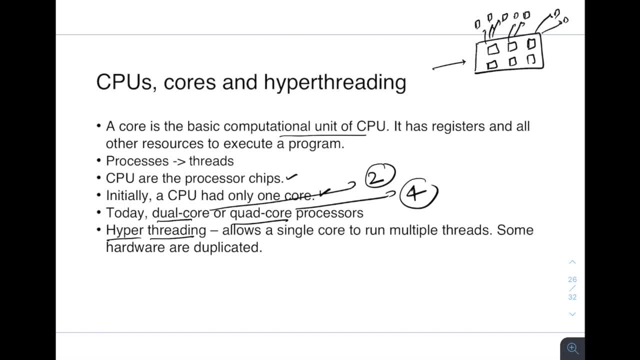 faster, I will say So. okay, now what will happen? Let's say, if you have four cores and you have also a hyperthreading enabled, then you can run four into two threads at the same time. So that's the advantage of using hyperthreading. If you do not have hyperthreading, then each 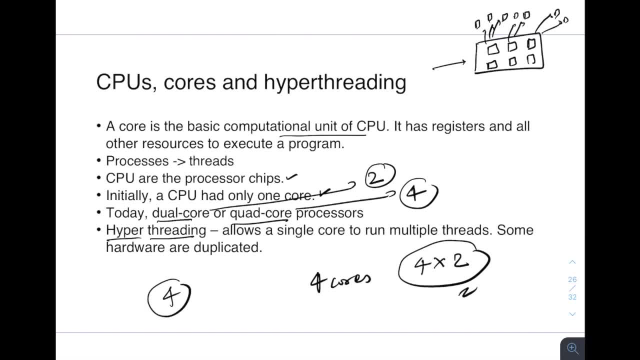 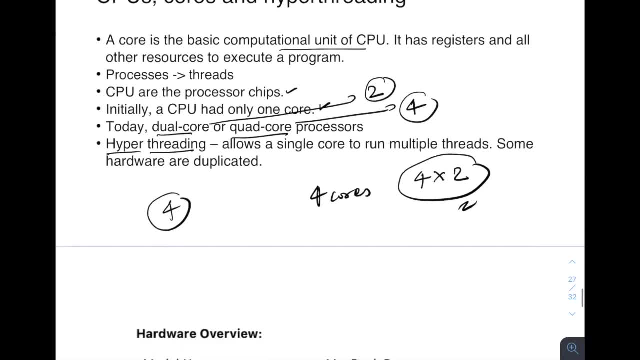 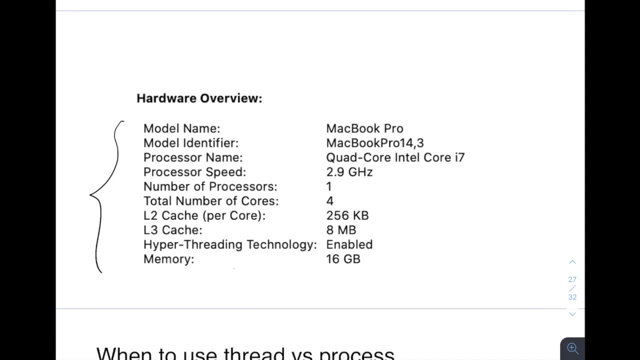 of these four cores will only run like four threads. Understand this. So basically, hyperthreading, you get additional resources for running threads. I'm not discussing this in details. You can maybe Google it and understand it more. So this is the hardware overview for me. So if 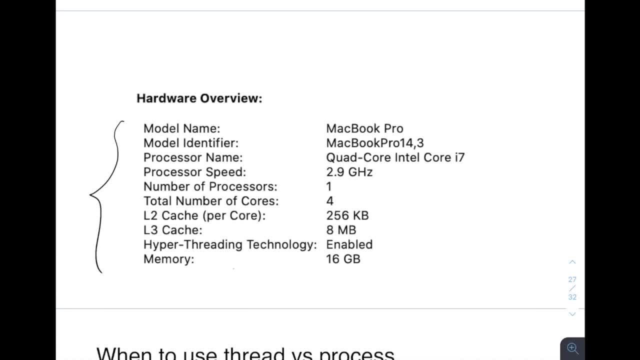 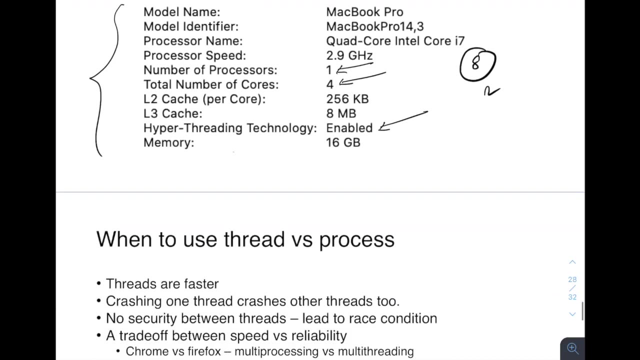 you see here, the important thing is here The number of cores, number of processors. of course I have one processor chip. The number of cores is of course four in that and hyperthreading technology is enabled. here run eight threads at one go in this because of hyper threading is enabled. now this is a debatable 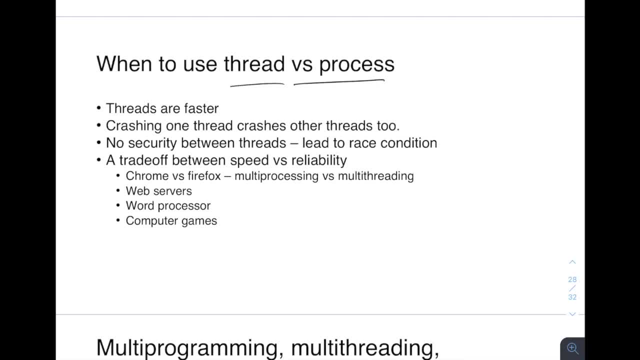 thing like when to use thread versus process. so threads of course are very faster than process, but another is some. they have some disadvantage with threads. also, like crashing one thread crashes other threads. there is also no security between threads, because you saw that right in the that example. it led to race condition when multiple threads were trying to update the. 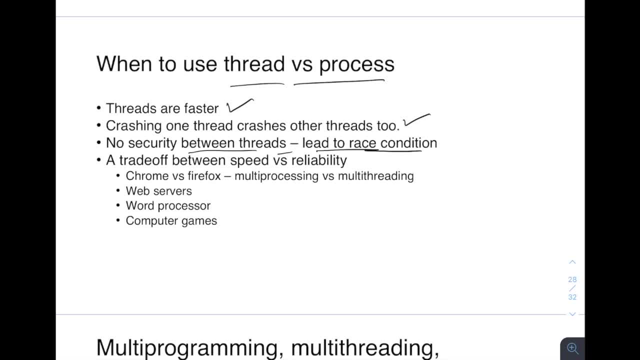 same variable at the same time. so of course you have you all always have to do a trade-off between speed versus reliability. so these two conditions are not very reliable. right, it is, makes your program more unreliable, and but? but kids also increase your speed of your, of your, i mean, if 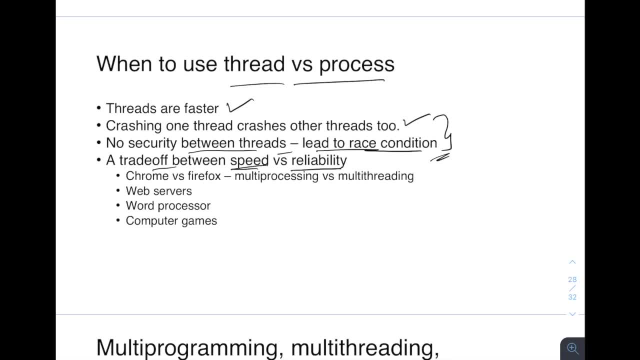 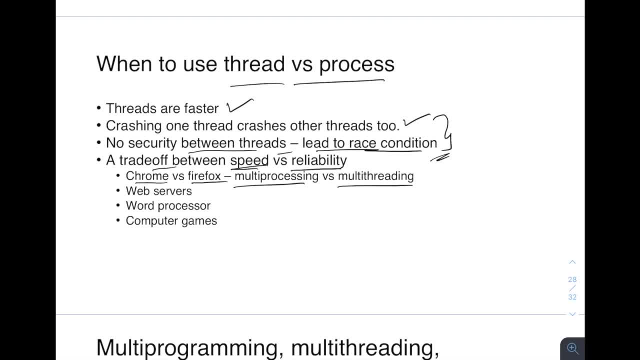 firefox in one thread crashes your whole firefox will basically hang in chrome. it does not happen. but chrome normally, you will see it uses, consumes a lot of your memory and cpu. you will see that. just open the chrome, five chrome tabs and see like how much uh, this chrome processor are using your. 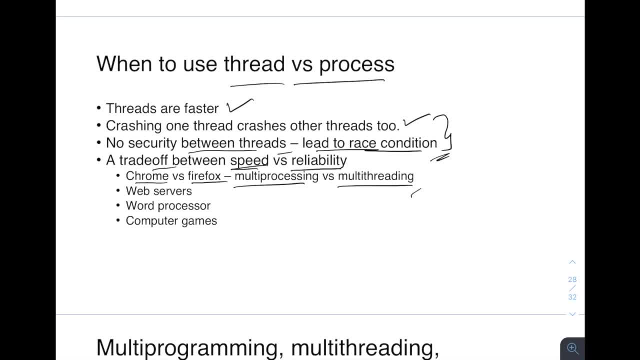 resources. you will see that. open five firefox tabs which are using multiple threads and see the resource utilization. you will see the difference there, of course, but in web servers- word processing, computer games, which need to be very fast, like the response time in this, needs to be very fast- in this case, mostly multi-threading will be more beneficial. so let's understand between. 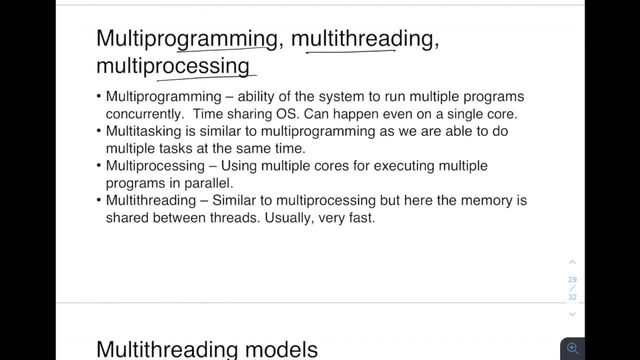 multi-programming, multi-threading and multi-processing. this is just the last part coming to last 10 minutes. multiply, multi-threading and multi-processing. so multi-programming is simply ability to run multiple programs concurrently, right, even if you have a single code, you can. you can have multi-programming. 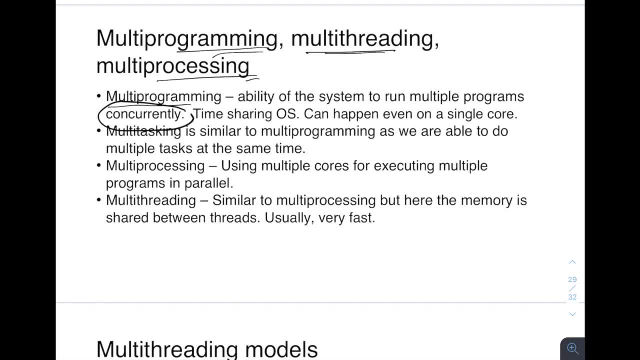 because i am discussing- this is important- concurrently. it is it? i mean it should not be like: okay, all the program are running parallelly, but they should be running very fast. like i can switch between very fast between chrome and text editor. i can also listen to music on my system. i can do all. 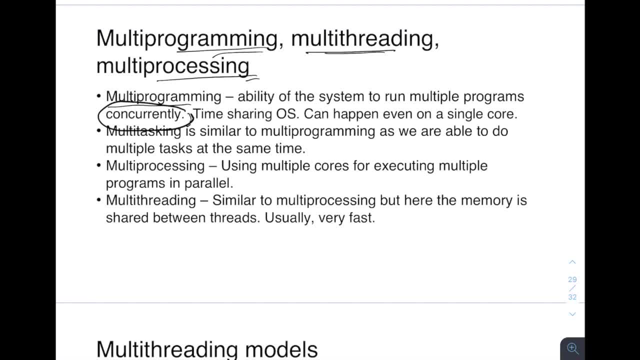 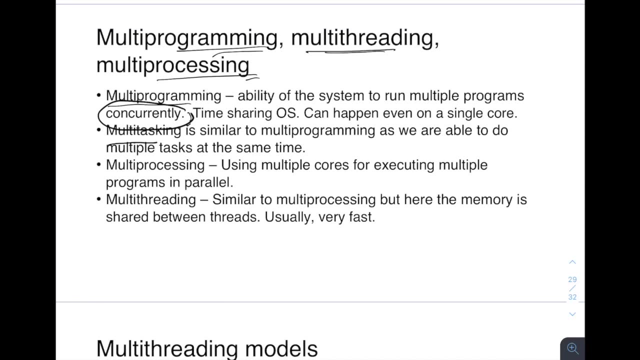 this at the same time. so if you have single processor, also through i mean round robin scheduling algorithm and context switching, this can happen. multi-programming can happen. multi-tasking is similar to multi-programming. in old times they used- i mean some everybody system called their processor as task, some will call them as process itself. so it is. 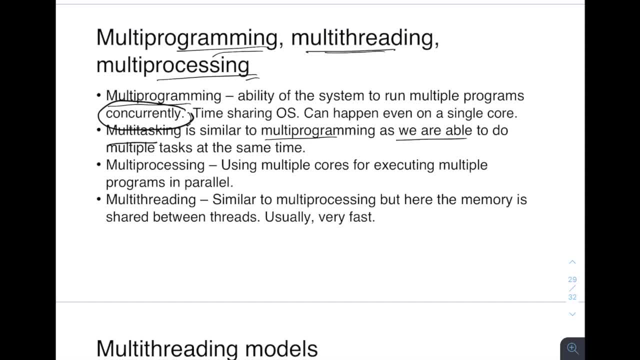 quite similar to multi-programming, because you are able to perform multiple tasks at the same time, right? of course multi-processing and multi-threading is different. of course, multi programing can use both of this if they want to: multiprocessing or multi-threading. but even if 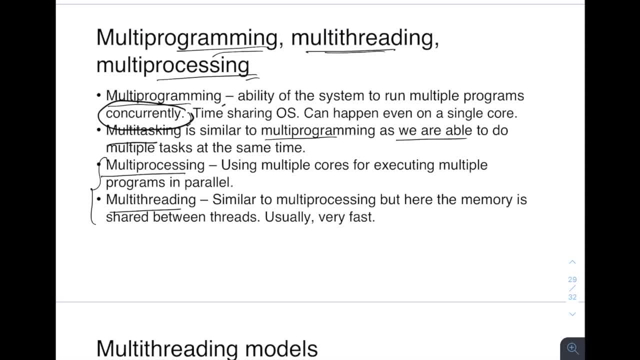 they do not want to use it. still, you can do multi-programming with the help of round robin scheduling algorithm. multi-processing is, of course, you know now, right using multiple codes for a single tool, right, you know you will. né executing multiple programs in parallel, right? multi-threading, again, is similar to multi-processing. 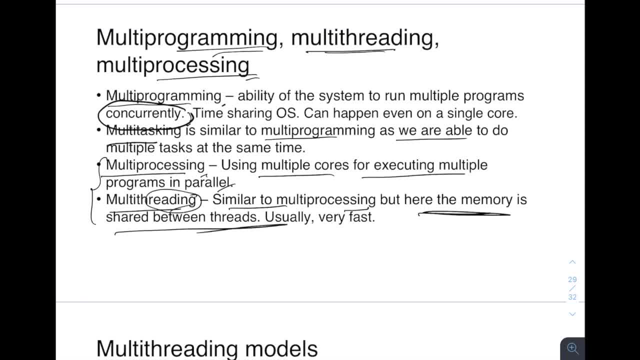 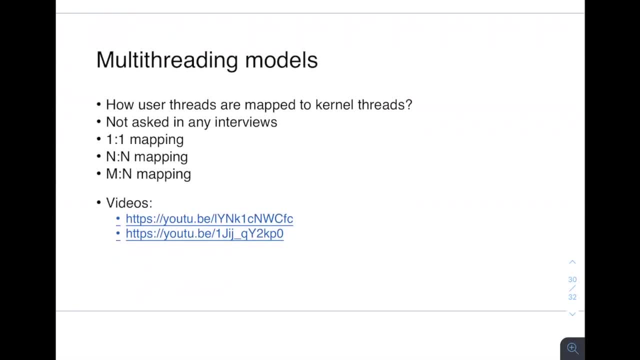 but here memory is shared. i mean, you're using threads instead of process and it's quite fast. uh, okay, multi-threading models. i'm not going to explain here. so there are three types of model, like normally, how the kernel thread, how the user threads are mapped to kernel threads.